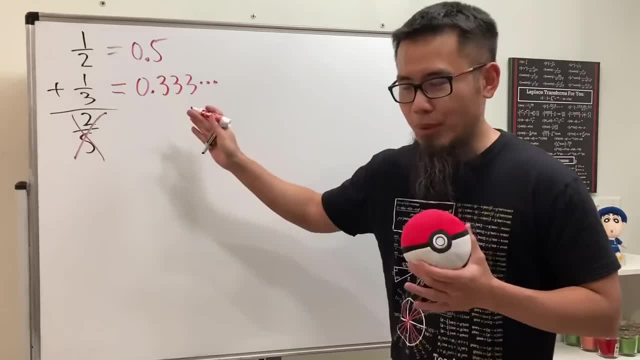 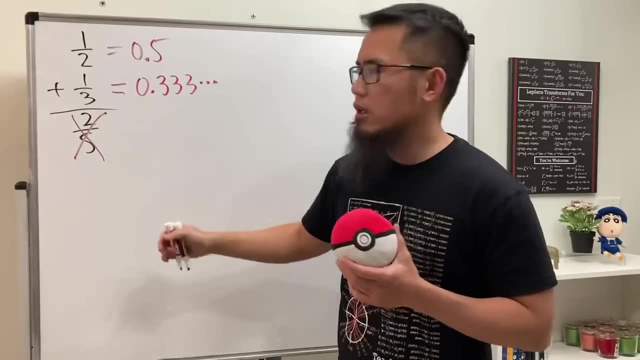 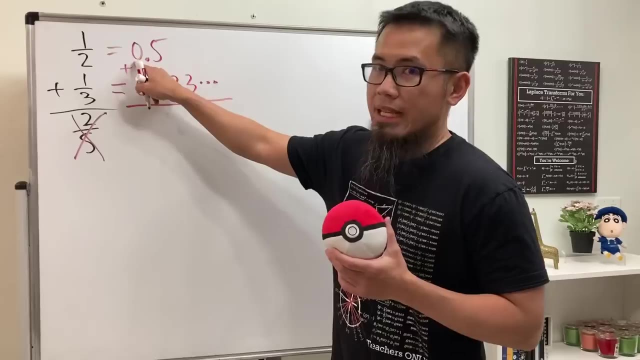 I know, I know it just feels being trodden, but I have my point right. Anyway, though, once you change the fractions to what we call the decimals, can we add them easily? Yes, you can add them very, very easily. Just go ahead and add them correspondingly right. 0 plus 0 is 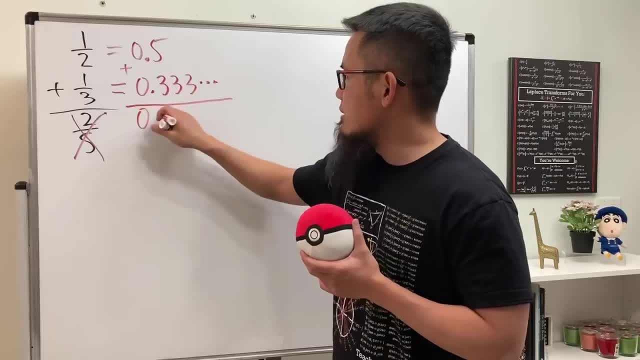 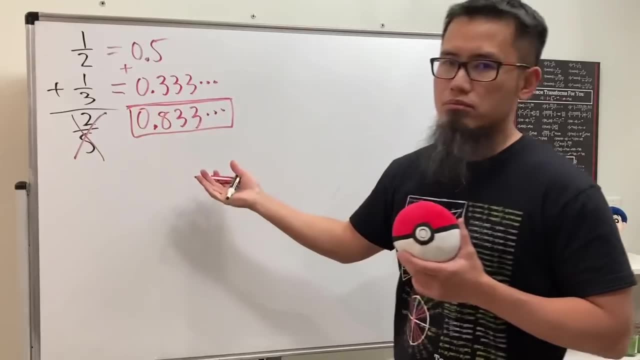 0,, and then 5 plus 3 is 8, and, of course, line up the decimal point, and then so on, so on, so on. And if you present this right here, wouldn't this be a legitimate answer? Yes, definitely right. 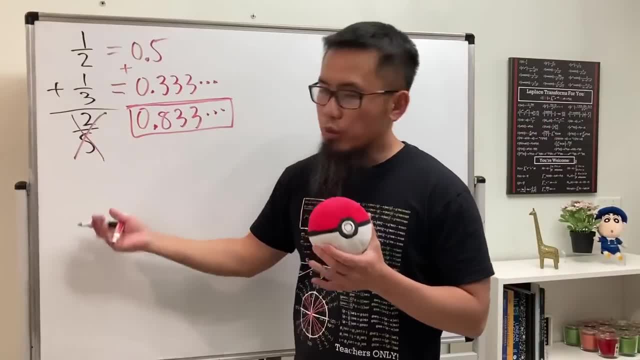 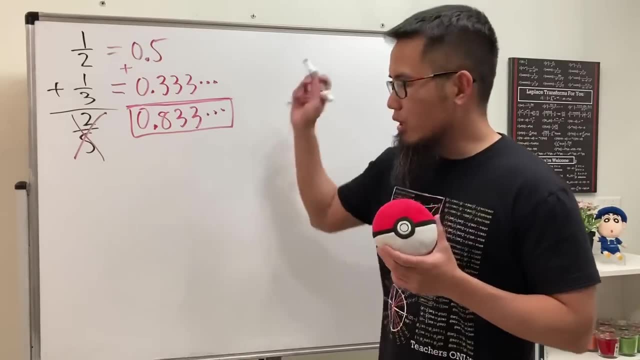 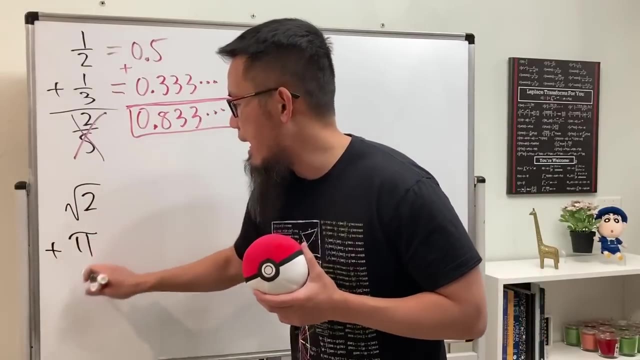 Now let me tell you, I think we just have been so used to fractions and decimals and we don't appreciate them anymore, And it's actually extremely useful. If you don't trust me enough, well, let me ask you what if we want to do square root of 2 plus pi? 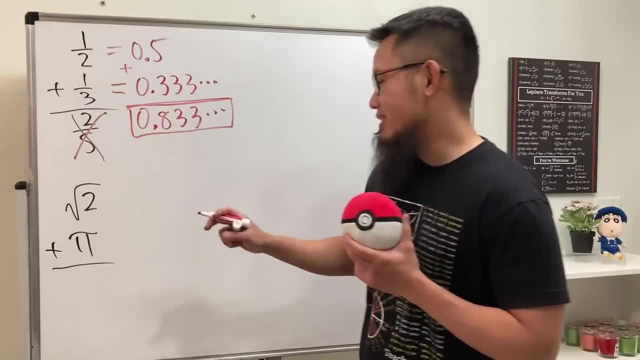 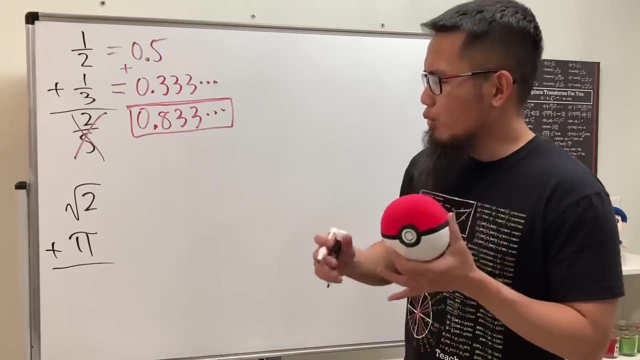 How would you do that? Ah, as you can see, I know, yeah, we're all good, right, Get a common denominator, things like that, But for square root of 2 plus pi, if you want to have a sense of how. 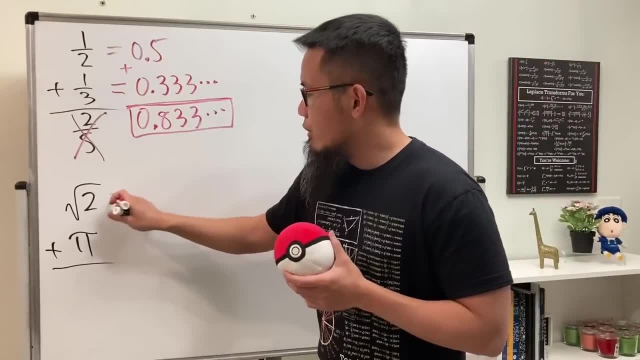 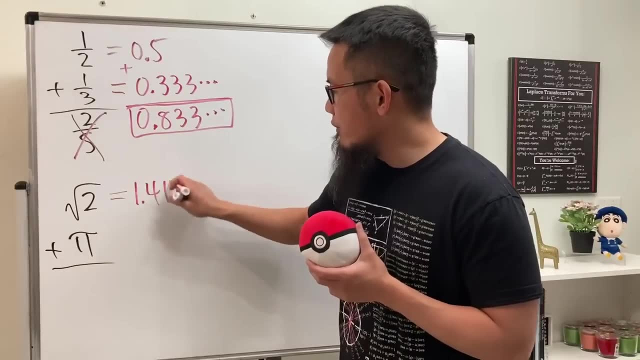 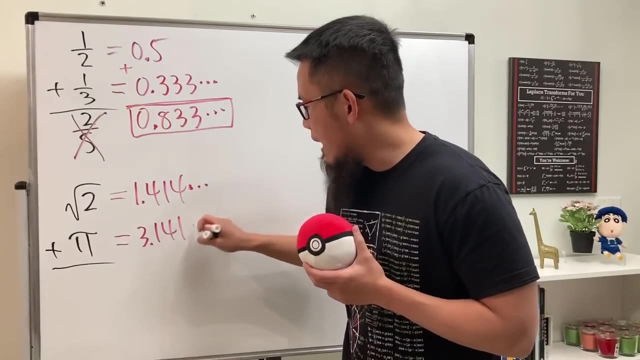 big. the numbers are right. the result is: well, we better change this into decimal and you will get the answer. So, square root of 2 is actually equal to 1.414,, and it actually keeps on going forever. And then for pi, it is actually equal to 3.1415926, and so on, so on, so on, right. 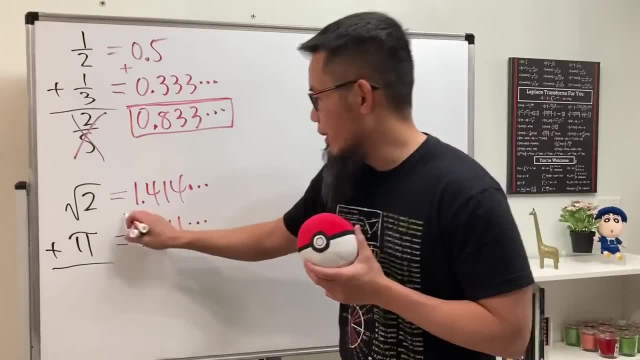 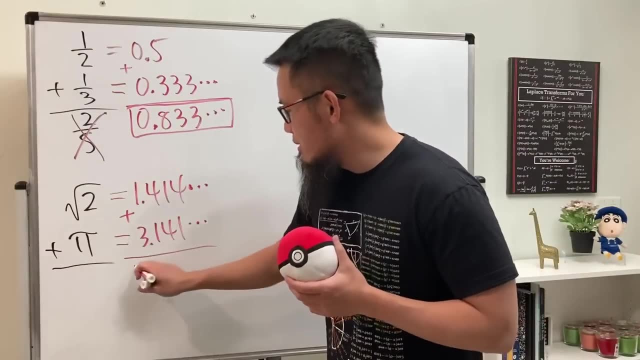 Anyway, though, once you change these two numbers into decimals, well, we can just add them up in a much more reasonable manner: 1 plus 3 is 4,, 4 plus 1 is 5,, and then the rest is just 5,, 5, and so on. 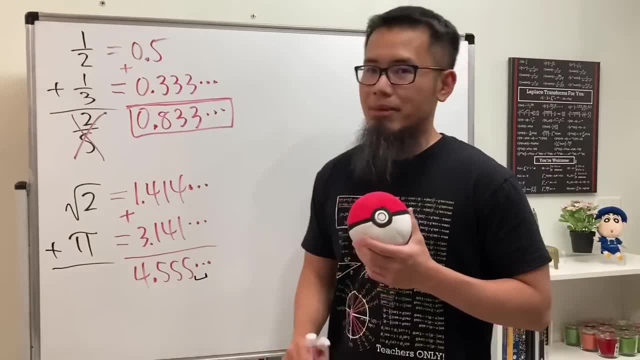 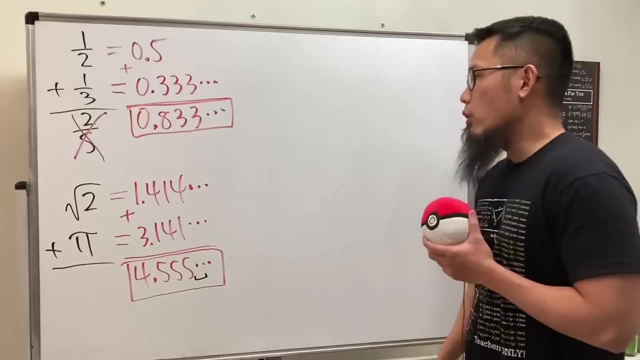 and so on. By the way, take a guess on what the next digit is. I'm not going to tell you. Anyway, this right here again, it's a legitimate answer, right? Good Well, I will tell you, guys some. 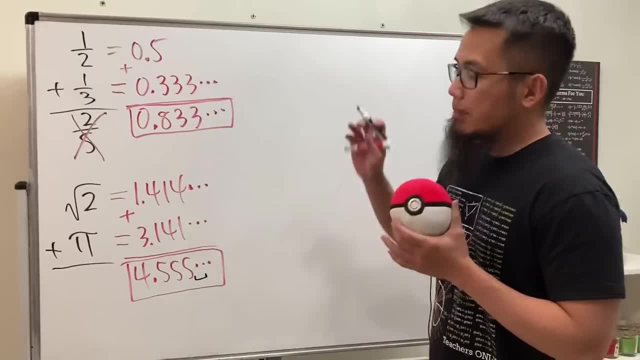 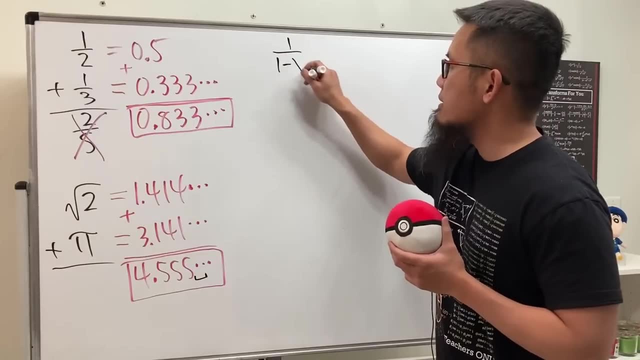 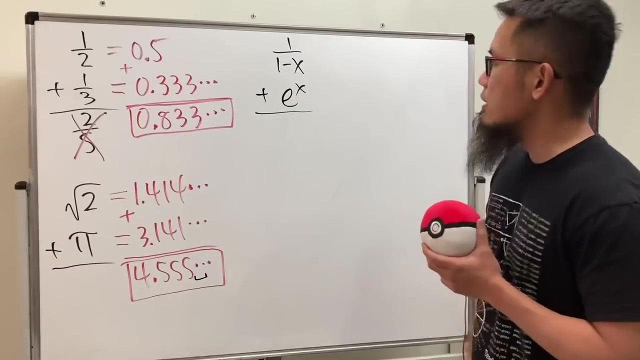 calculus things. Let's take a look at this right here. Suppose today we are dealing with functions rather than numbers. Let's look at if we have the function 1 over 1 minus x, and I want you guys to add it with e to the x. Of course there are common functions in calculus and uh. 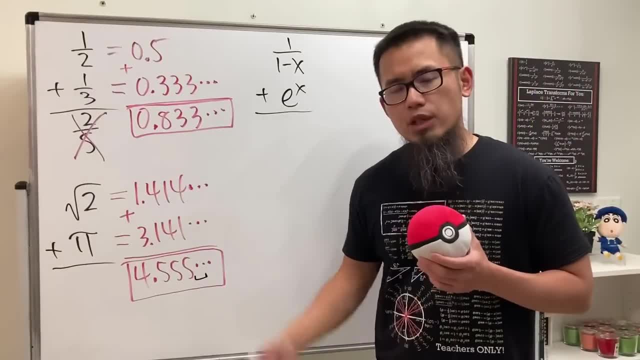 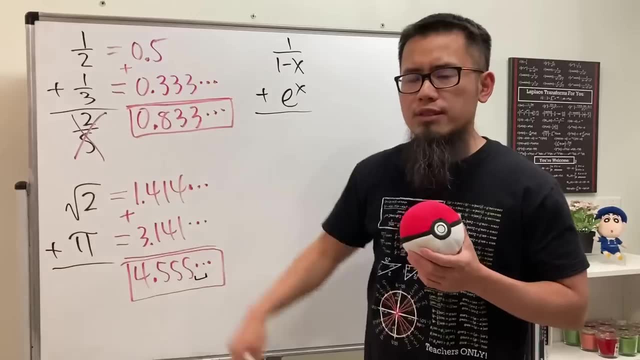 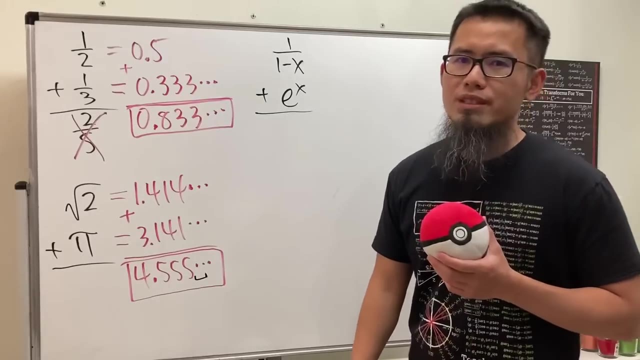 to add these two functions together. yes, we can just get a common denominator, But I don't even know how to get a common denominator with the regular fractions. You really think that I can get a common denominator for these two functions? Don't do that to me, But I will do this for you. 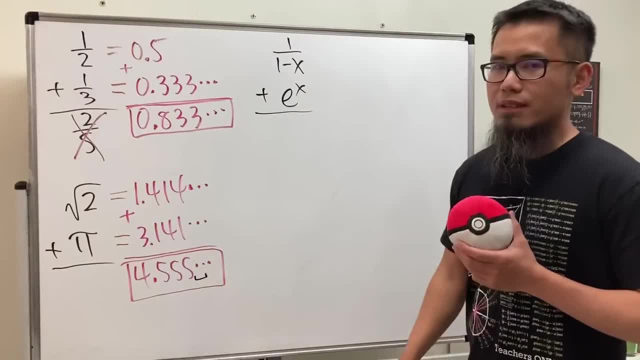 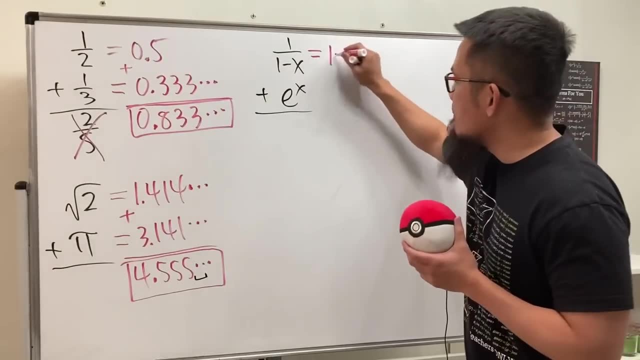 guys Check this out: 1 over 1 minus x, as long as we are willing to do some magical work and we can show that e to the x is equal to 1 plus x, plus x squared, plus x to the third power and so on. 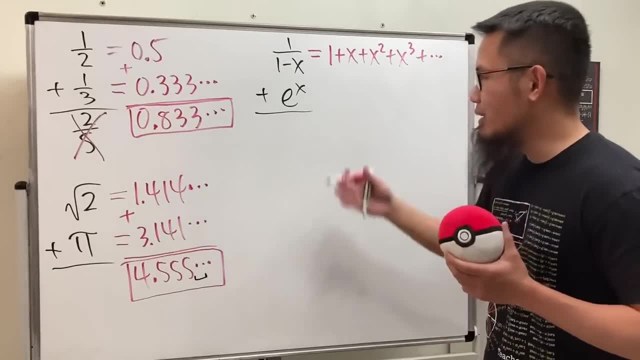 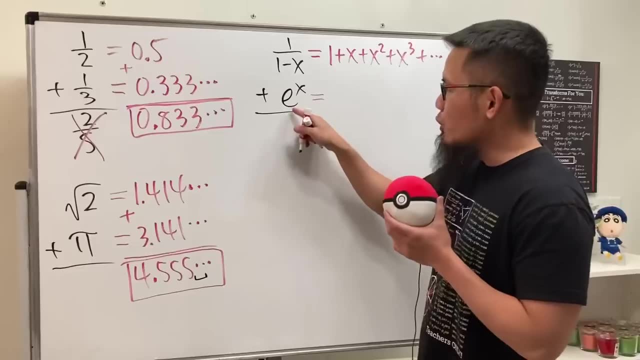 so on, so on. And, ladies and gentlemen, are you guys ready for the next one? Hopefully, This right here. as long as we are willing to do some magical work, we can show that e to the x is equal to 1. 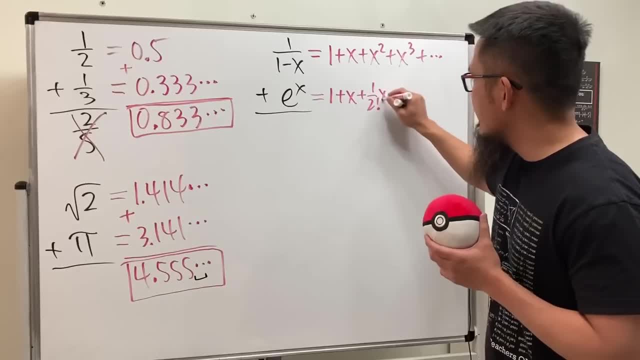 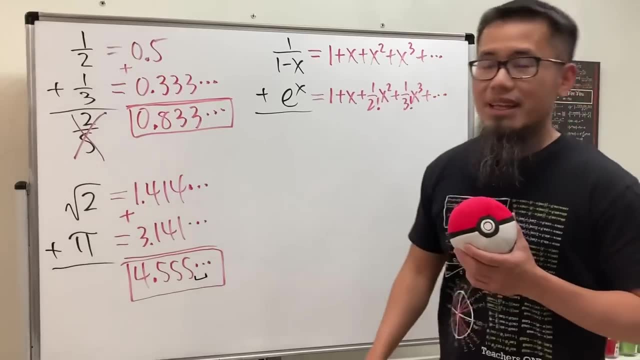 plus x plus 1 over 2 factorial, x squared plus 1 over 3 factorial, and then so on, so on, so on. Ah, Now, as you can see, we have a common denominator and we can show that e to the x is equal to 1 plus x, plus x to the third power, and so on, so on, so on. 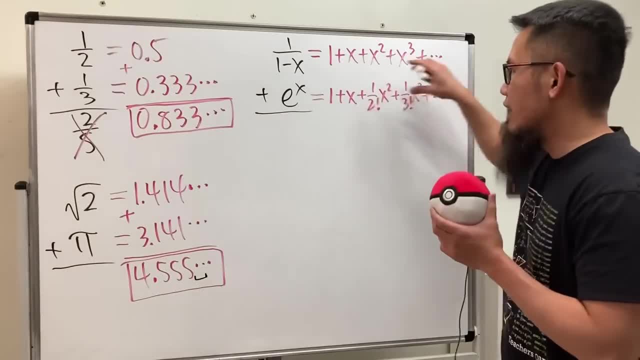 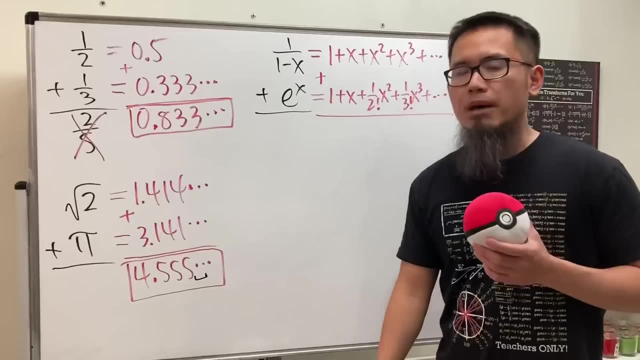 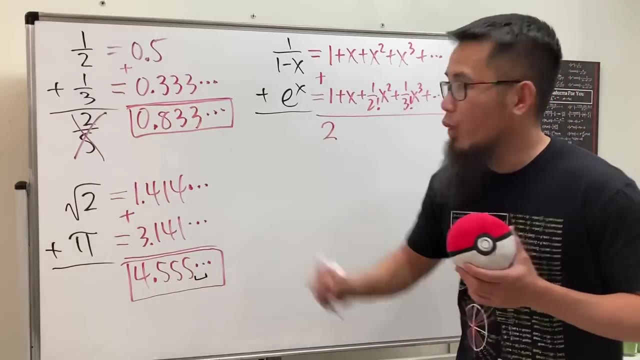 These right here are just polynomials, although they have infinitely many terms. But if you look at this right here and if you want to add them up, can we just add them up correspondingly? Yes, Check this out: 1 plus 1 is equal to 2, and we can do that legitimately. We couldn't do that with. 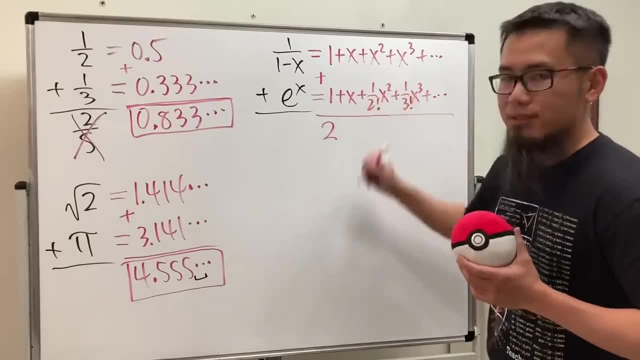 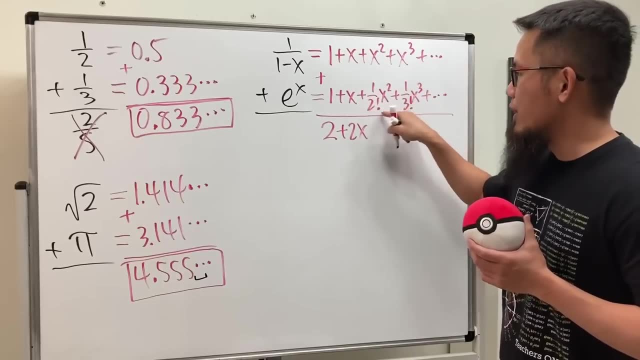 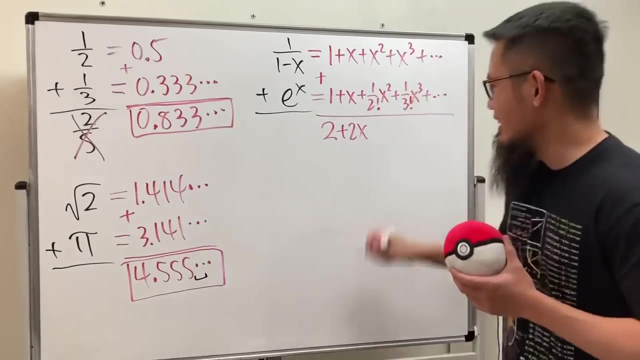 fraction earlier, Huh. And then for the next one, x plus x is 2x, And now this is 1 x squared plus 1 over 2 factorial, which is 2.. And then, yeah, 1 plus 1 over 2, give you a common denominator, okay, And you get 3 over 2 x squared. 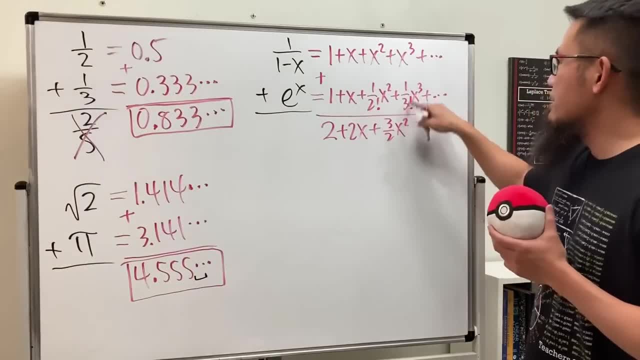 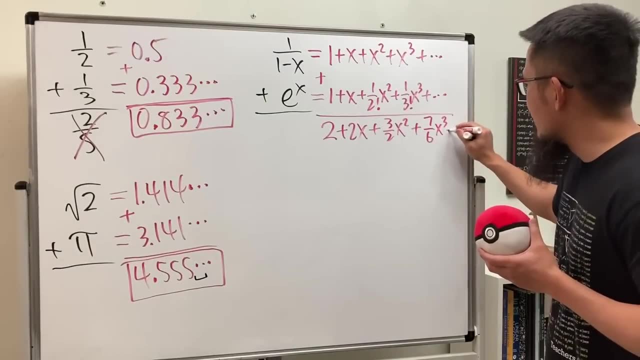 and then this is 1 over 6, right 3, factorial 6, and then plus 1.. Altogether again get you a common denominator. You will get 7 over 6, x to the third power, and then so on, so on, so on. 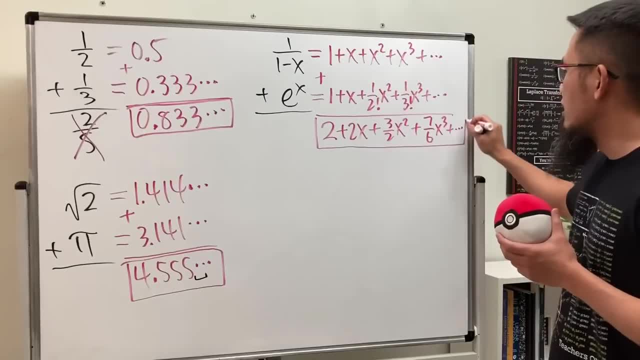 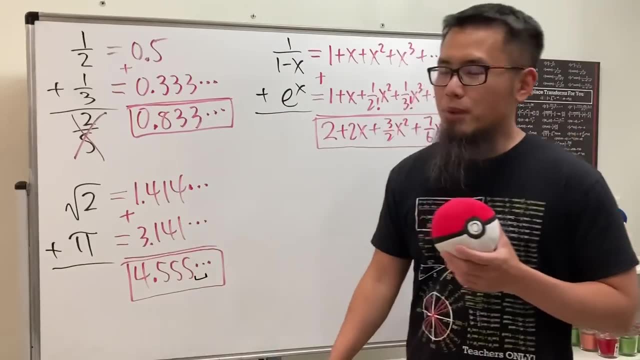 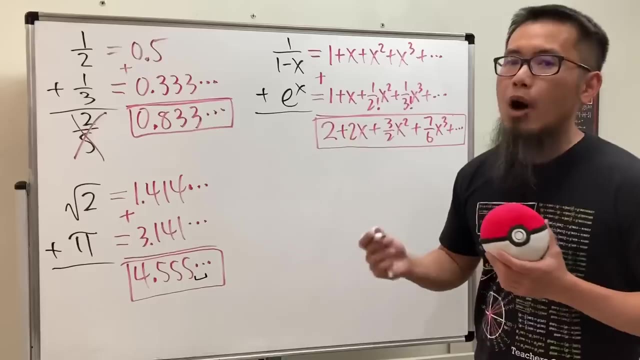 Well, again, this right here would be a legitimate answer, isn't it? Yes, definitely So. over here, I pretty much just used the decimal as an analogy to show you guys what this is all about. These right here are called the power series, And of course I will write that down. 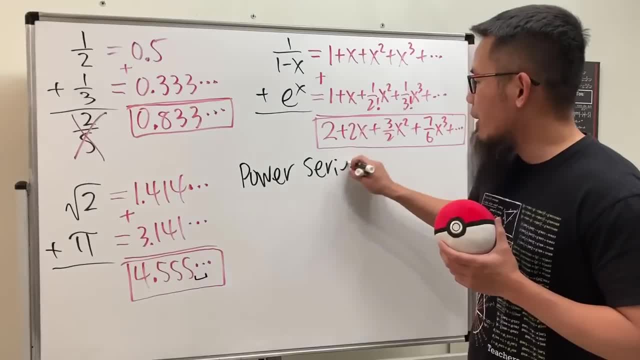 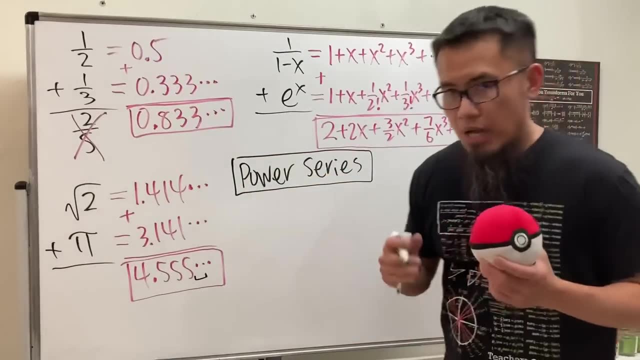 right here for you guys, And in fact, this is how I introduced the concept of power series to my calculus 2 students, right? So have a look. right here I want to tell you guys what power series is all about. As you can see earlier, decimal numbers make the computation so much easier. 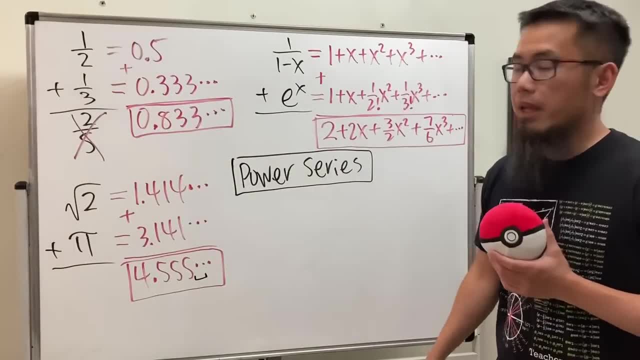 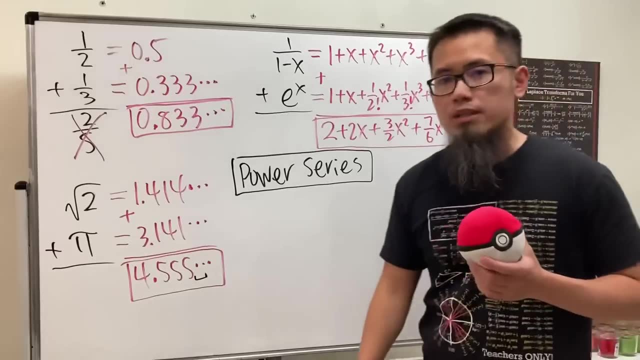 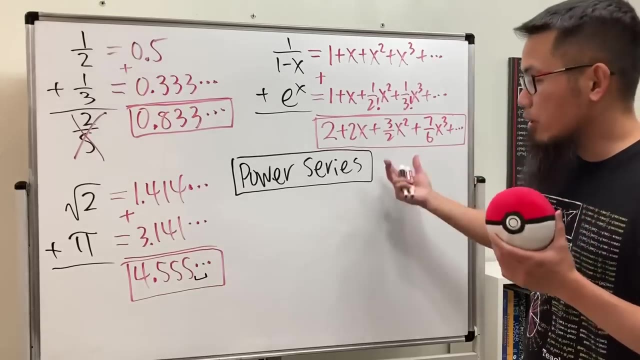 well, that's what power series will do for us as well. They will make the computation so much easier for us, Like, for example, in this case. but let's talk about calculus When we have polynomials, we love to do this right. We love polynomials because we can differentiate them. 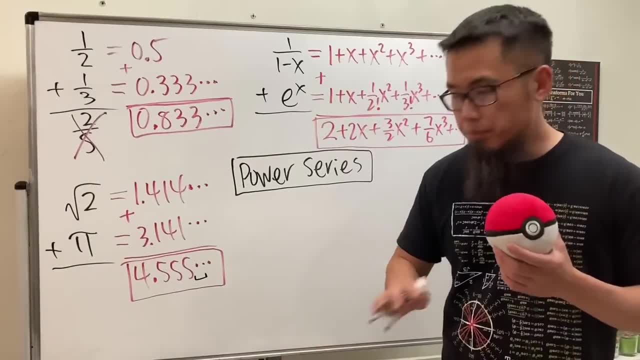 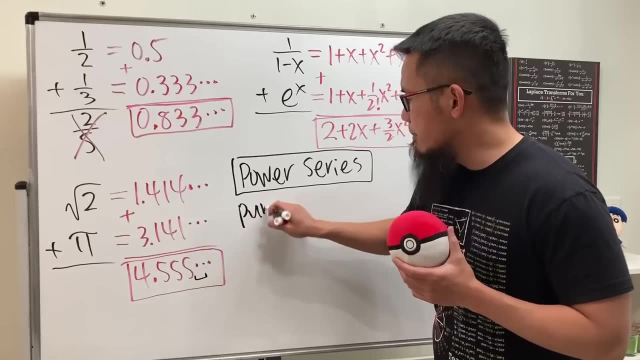 We love to integrate polynomials because they're so much easier. So the goal for the power series is the following. So let me write that down right here. This is the purpose or the goal of power series. As you can see, on the left-hand side we have 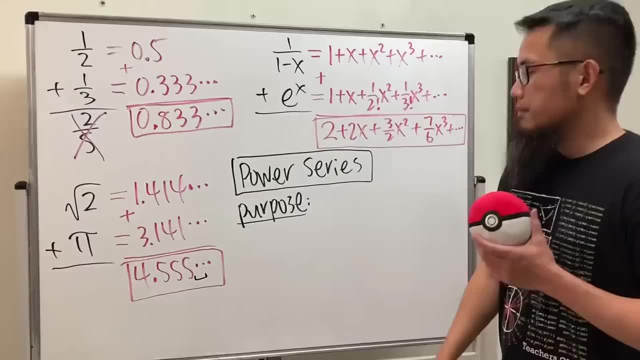 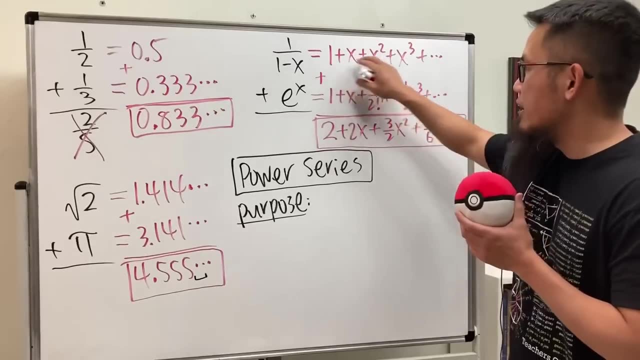 functions that we might not like too much. I will consider these two as that complicated function, but on the right-hand side we have infinite polynomials because they have infinitely many terms And they are polynomials because you see that we have x to the first power, x to the second. 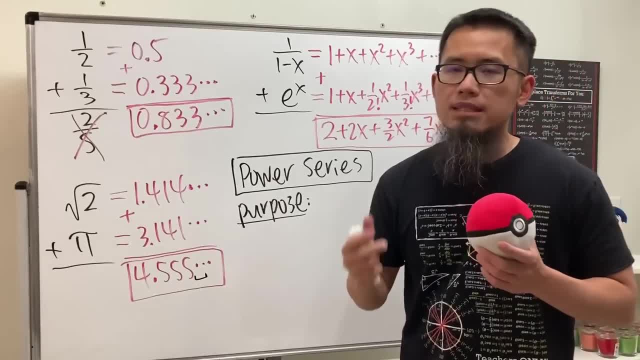 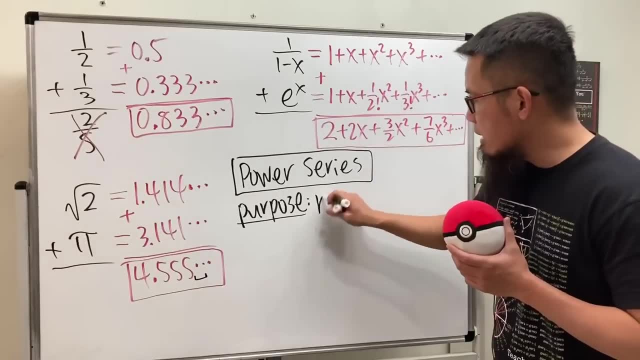 power and so on, All the powers of x. they are just positive whole numbers And of course we have the constant terms. So the purpose of the power series is that first we will represent, and I'll just say they are. 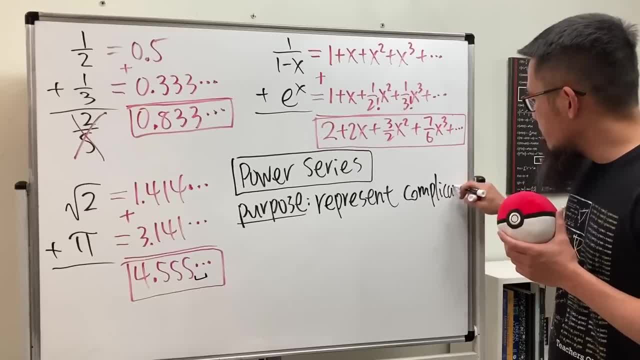 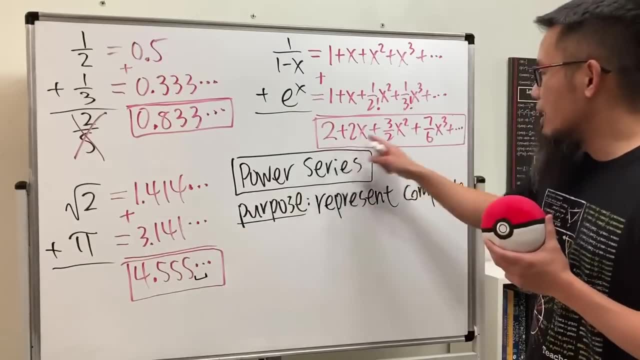 complicated functions. And what do I mean by complicated? Anything that's not polynomial I will consider to be complicated. Because if you look at a polynomial, if you want to differentiate or integrate them, you can just use the power rule. How cool is that, right? 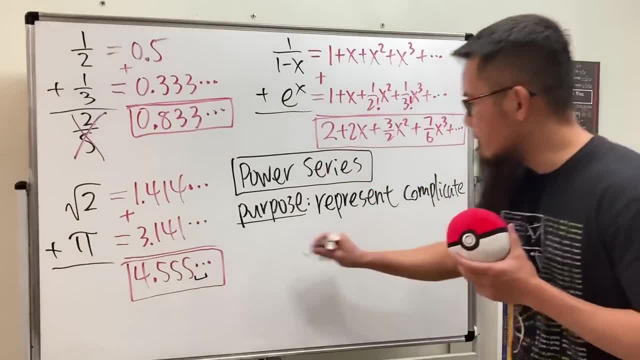 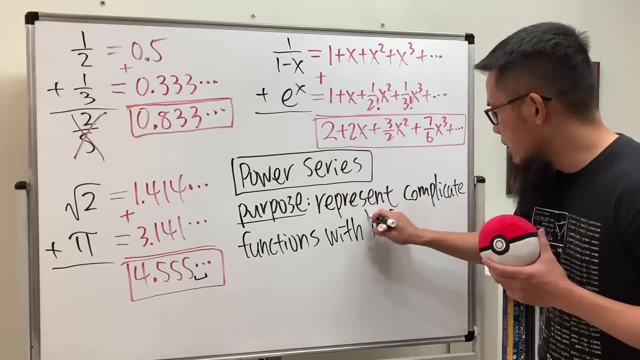 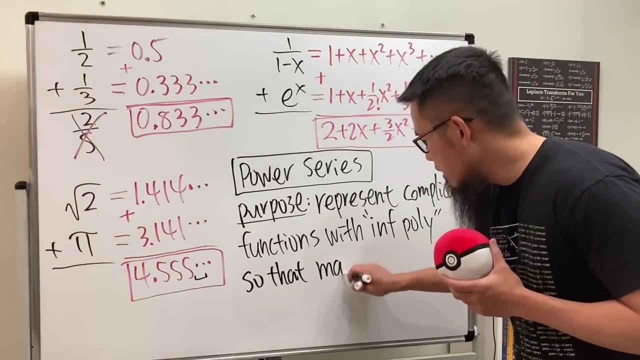 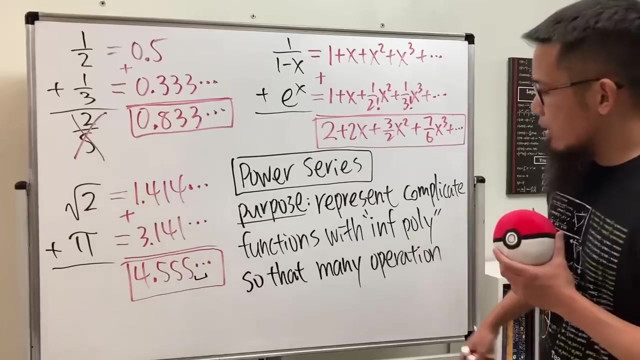 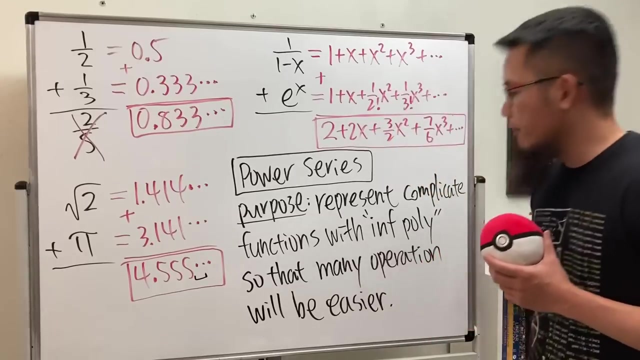 So the purpose of this is to represent complicated functions with infinite polynomial so that- and I will just tell you guys the following, many operations, or maybe, if you want to do approximations, all right, will be easier. That's pretty much the idea. 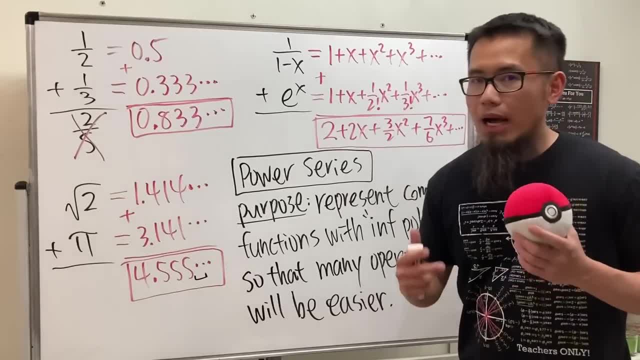 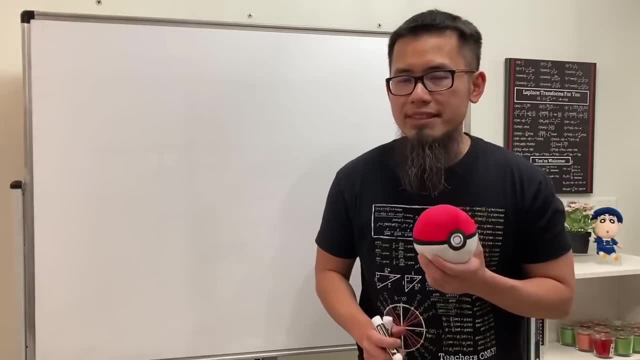 Again, just take a look at this right here And now. I would like to tell you, guys, what are the things that we'll be doing for power series. First, let me tell you what are the things that we need when we are working with power series. So right here, the first thing that we need. 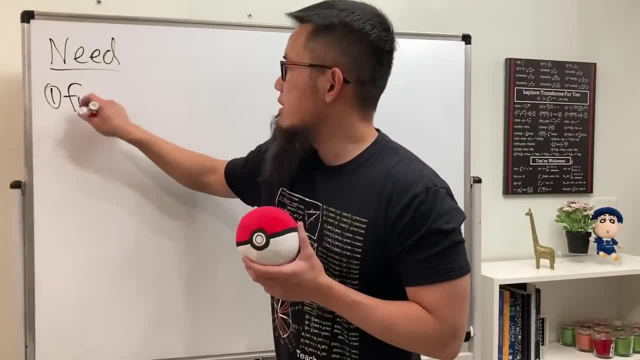 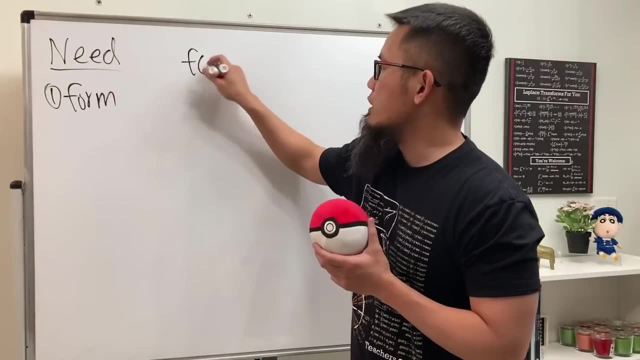 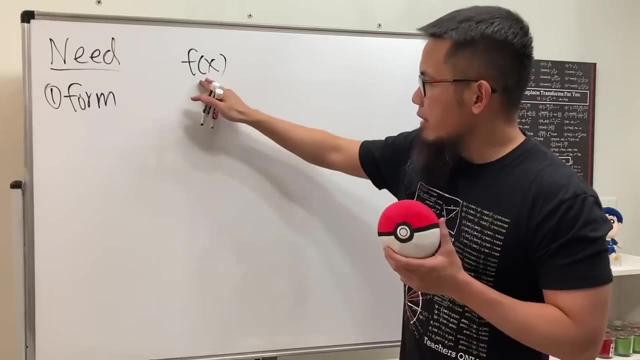 I will call that to be the form of the power series, And that's just simply how the power series look like, right? So remember earlier we were talking about when we have a power series. we are trying to write a complicated function denoted by f of x in general. write this as an infinite polynomial. 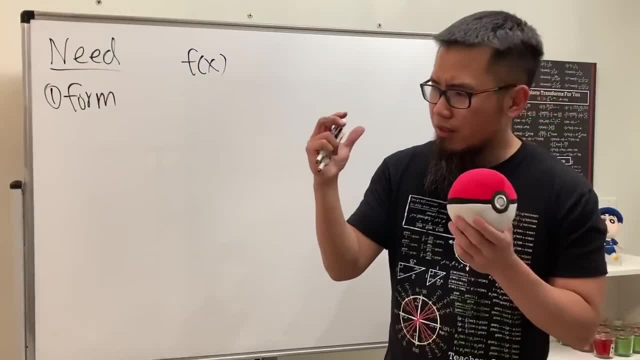 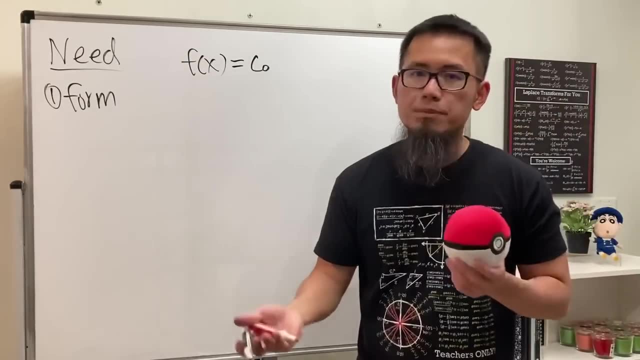 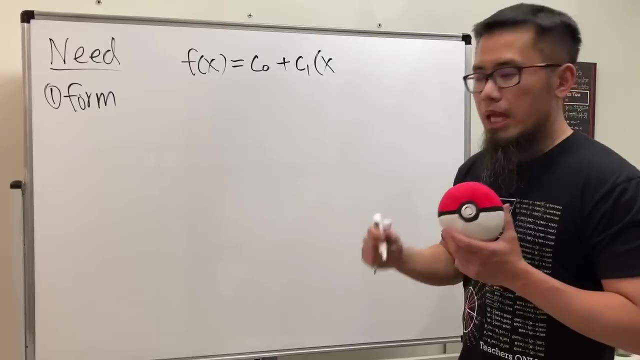 And when we have an infinite polynomial, we have the constant term And the notation for that is c0, and then next we have the x to the first power term, And it has a coefficient as well. so we'll just put down c1 times x to the first power, But in general we may have what we call. 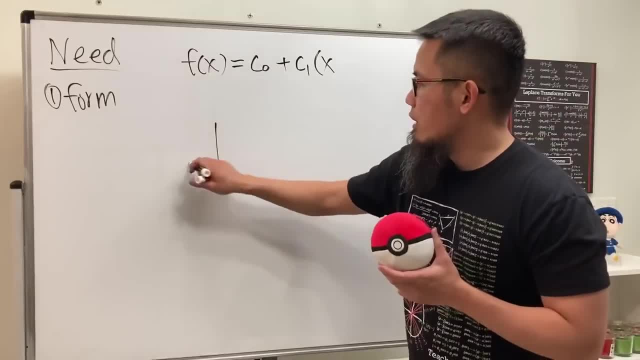 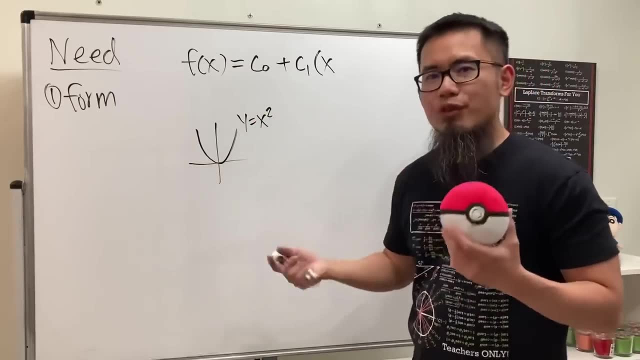 the difference center. What I mean by that is the following: Well, this is our girlfriend. right. y is equal to x squared, But we can move this around. it will have a different center, right, Suppose I move it to here. let's say this: right here is 3.. 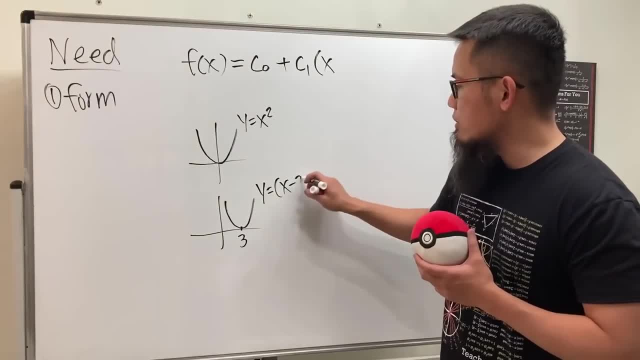 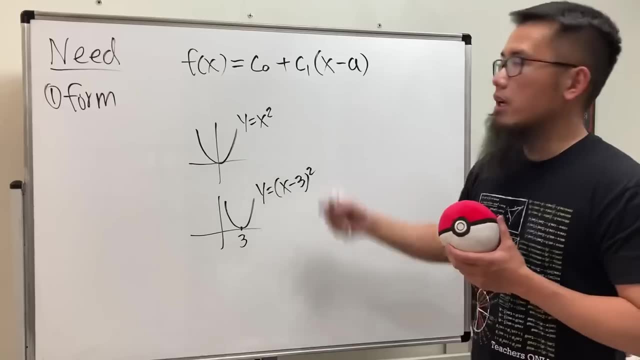 Then in that case the equation becomes: y is equal to x minus 3 squared. So in general we'll write this as x minus a, and then to the first power. So we'll use this as an input in general and the a is called the center, And then next: 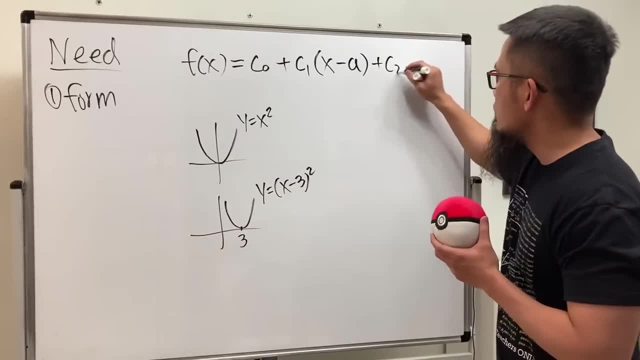 we have the x minus a and then to the first power- So we'll use this as an input in general- and the a is called the center. And then next we have the second degree term, where c2s is the coefficient, and then x-a to the second power, and then so on, and so on. 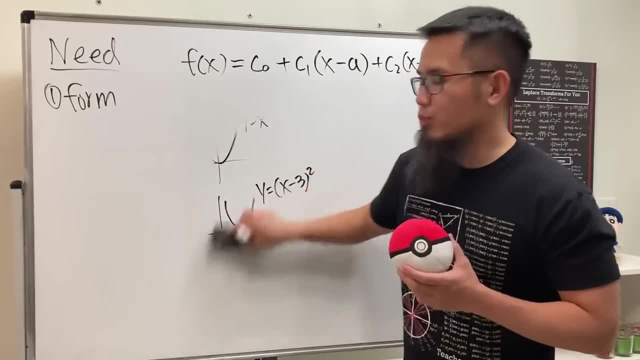 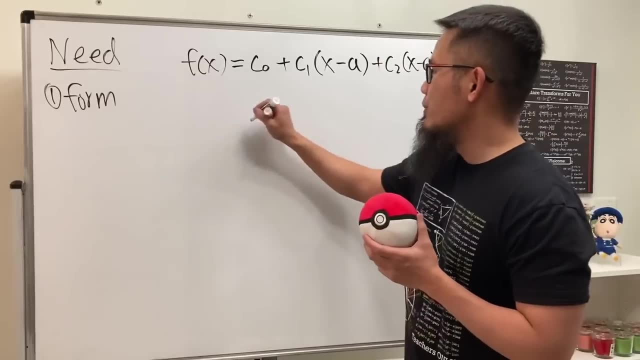 just like that. Off course, that is a lot to write. We don't like that. It's OK because we can just use the sigma notation for it. So to put this in the sigma notation, it will be the series as n goes from zero to infinity. 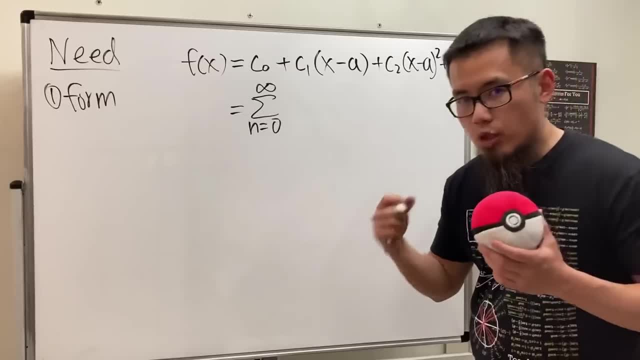 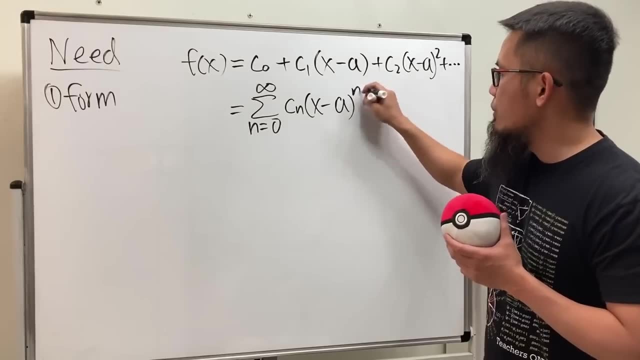 All the c's right here are the coefficients. so m goes from one to minus 1.. So we just add all the functions and write this down as cn, and the input right here is the x minus a to the nth power, like that. so 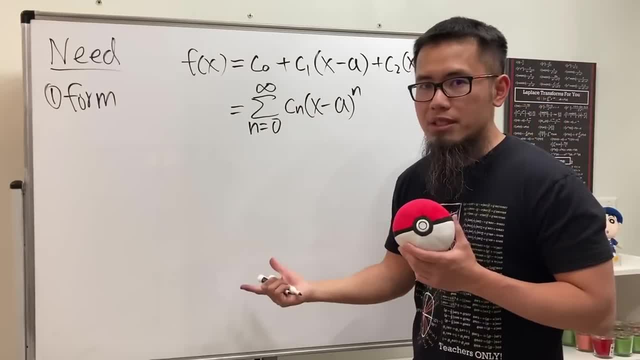 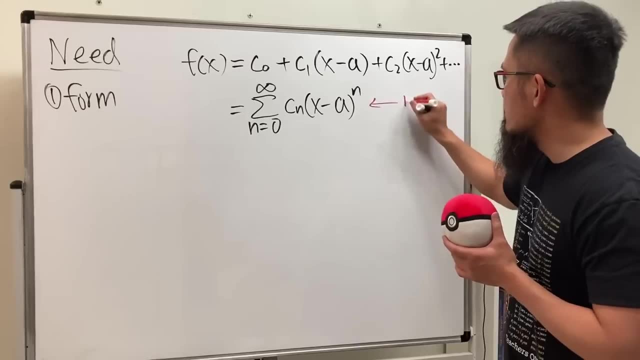 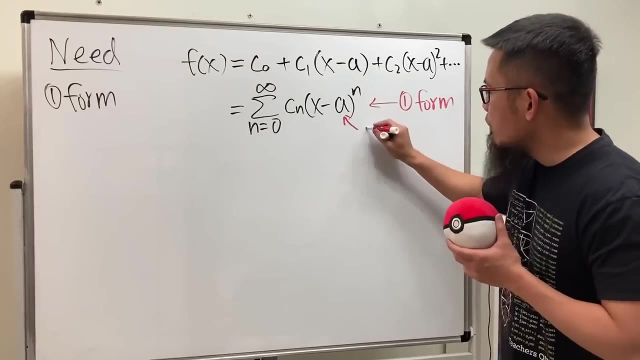 this right here is what i call the form of the power series. it's just simply how the power series look like. let me write that down real quick. this is the first thing. this is just the form and, just like i mentioned earlier the a right here, it's called the center of the power series. 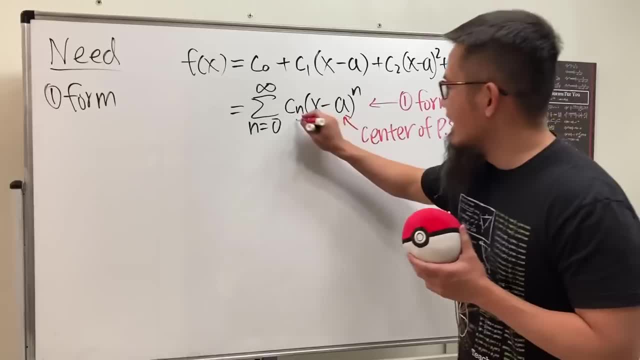 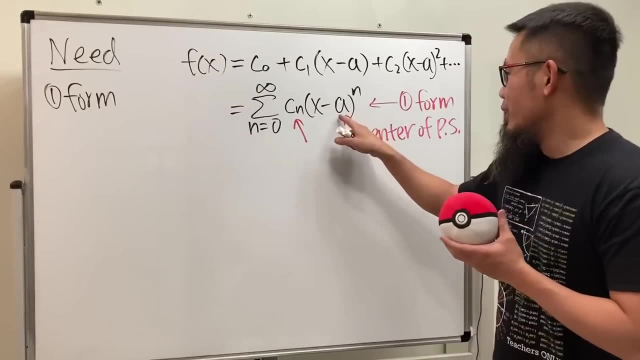 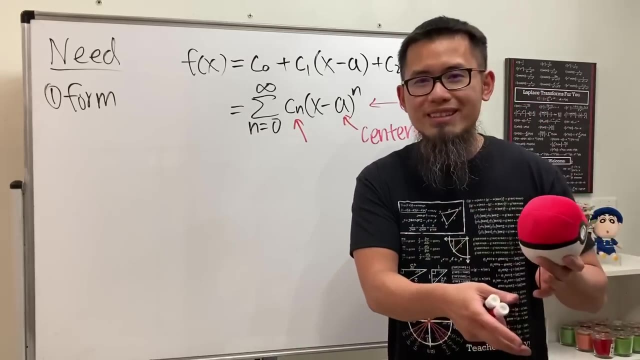 ps, not playstation, right, power series and the cn right here, which is actually the hardest part to find out, because for the center you just have to wait for the direction. okay, find the power series at a is equal to whatsoever, right. so this right here is usually given. but for the 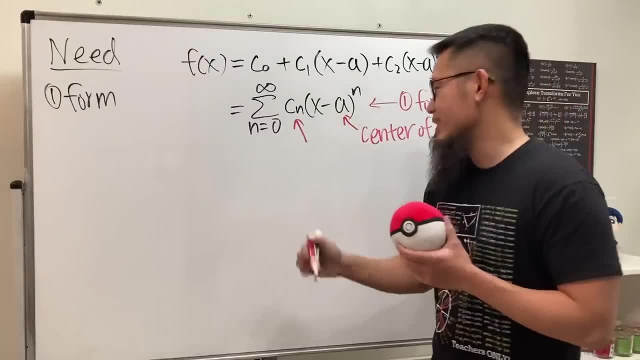 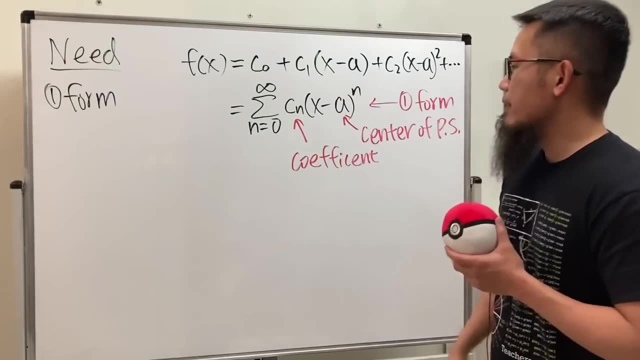 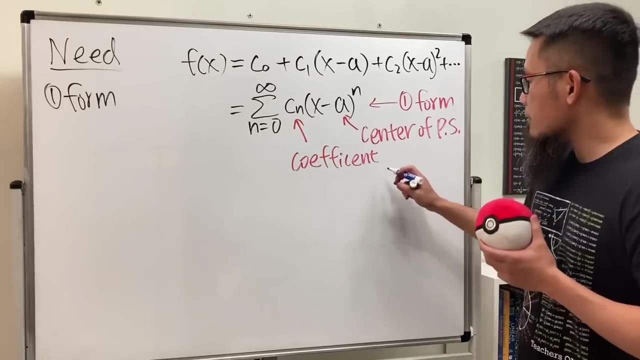 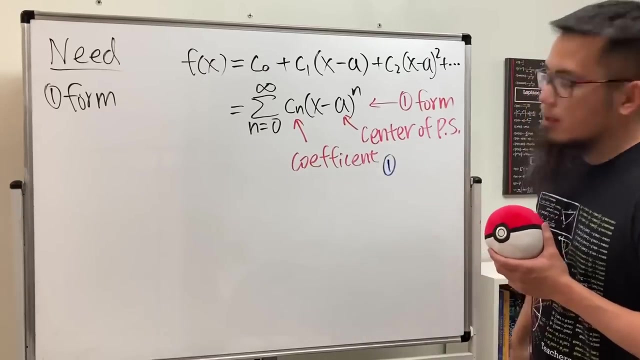 coefficients. you will have to do some work to find out, so let me write that down right here. so let's say we have the coefficients, right. so how can we find the coefficients? um, i will tell you guys this right here, right for the form in general. we have two ways to do it. this first way is we are going to use 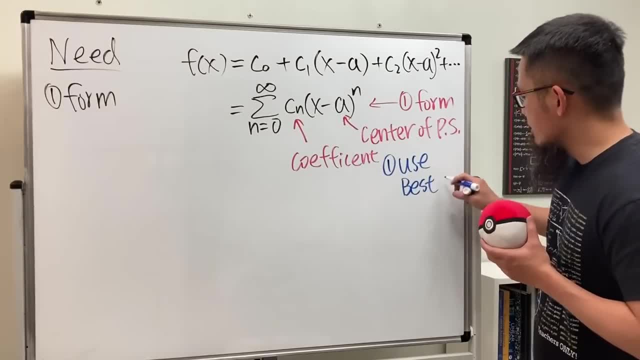 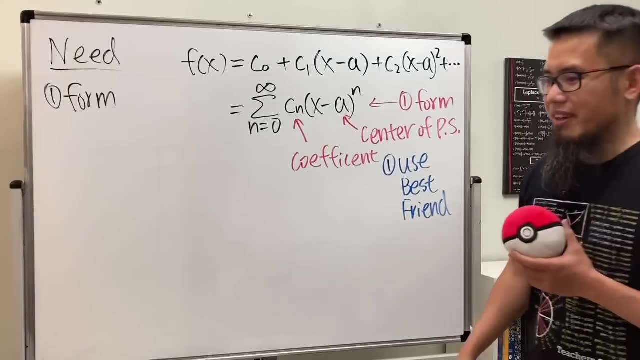 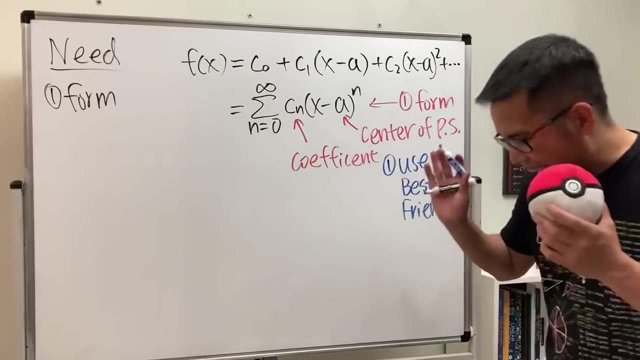 right what i call the best brand, best friend, right? so what's the best friend? just how i mentioned earlier, how can we find the best friend, use it? i will show you, because if you have a best friend, you should know how to use it. i know it sounds so bad, but math is totally okay. 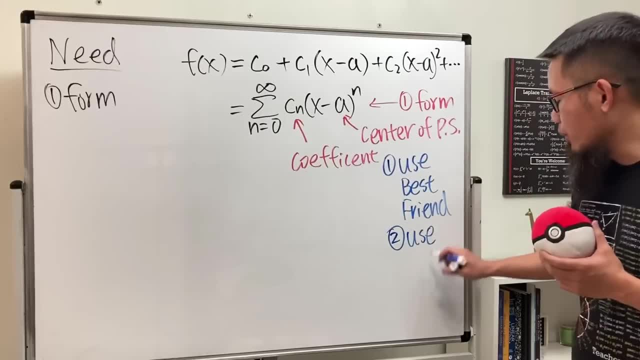 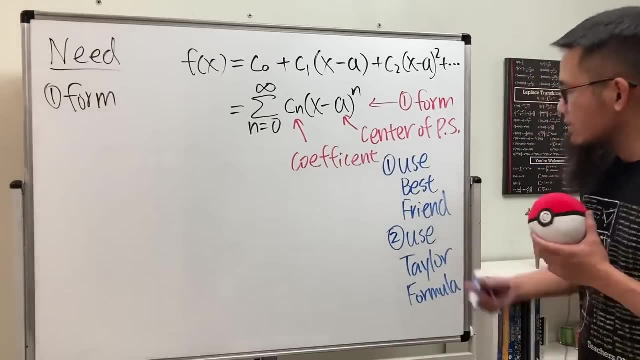 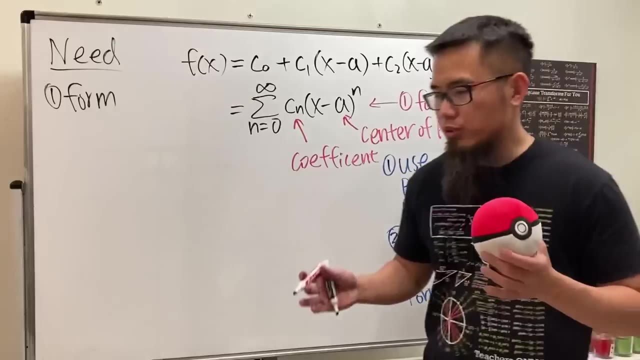 or the second thing that we can do is we can use what we call the taylor formula. what's the taylor formula, you ask? well, that will be later on. in fact, i'm just. this video is just to introduce you guys what power 3 is all about. i'm just going to show you guys what power 3 is all about. 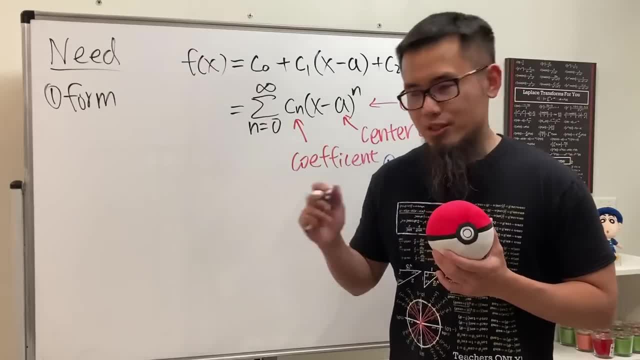 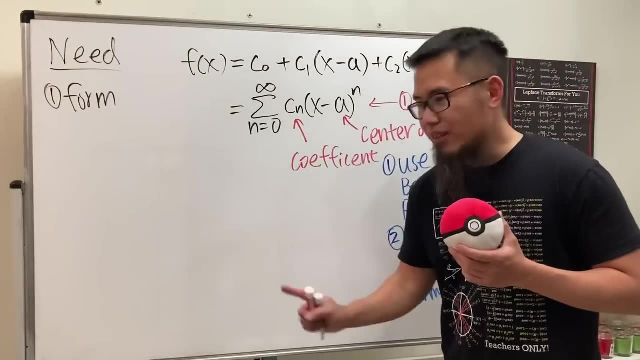 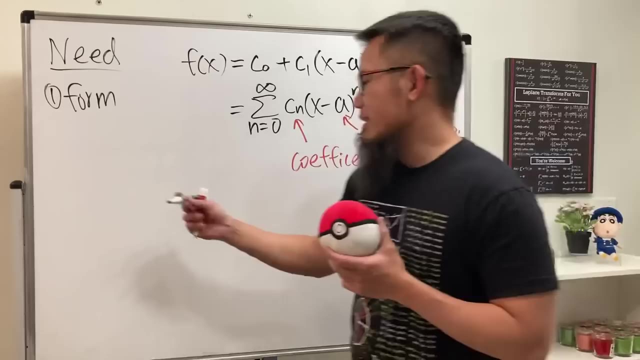 i have done a power series marathon for you guys already, so i will have that link to the in the description for you guys. i worked out 26.2 power series. after the video, you should be an expert on how to find the form and then the two other things that we need. all right, so that's the form in general. 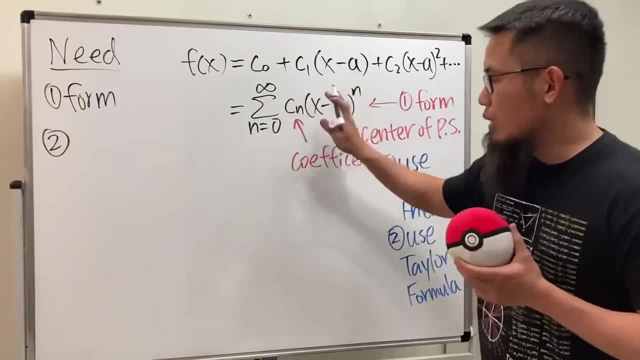 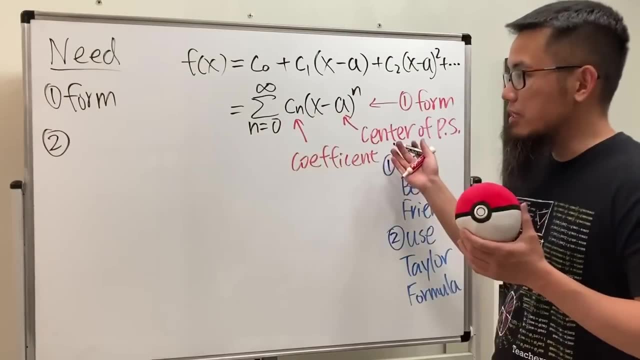 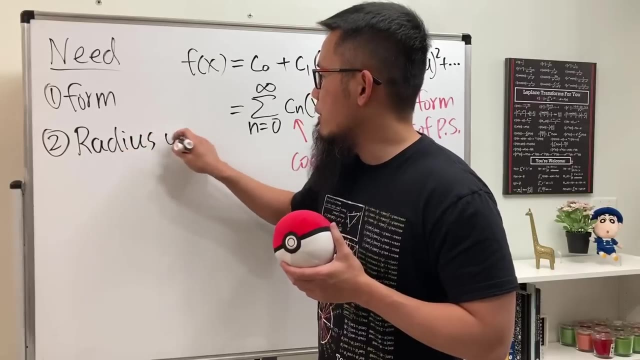 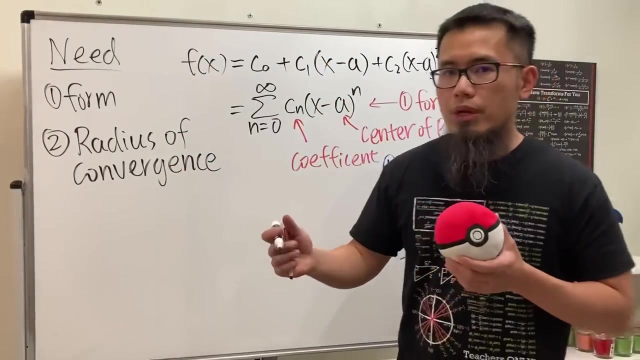 next, we need to know because when we have a power series, sometimes we might not be able to plug in any value using certain x values because there are restrictions. those restrictions came from what we call the radius of convergence, and this simply tells you how far you can go out away from the center. so when you have the form, 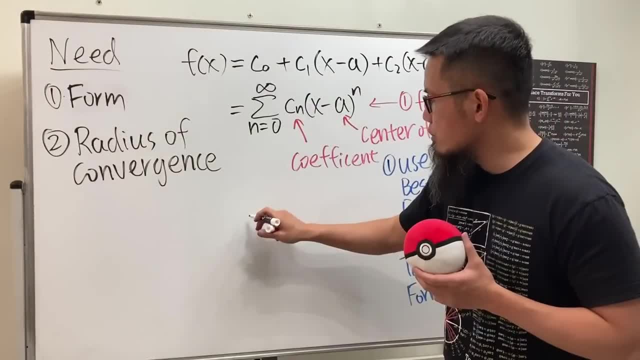 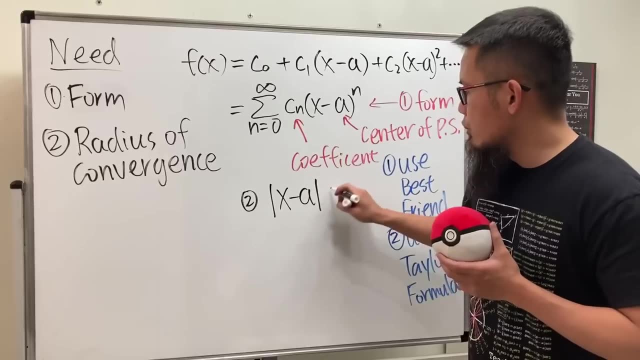 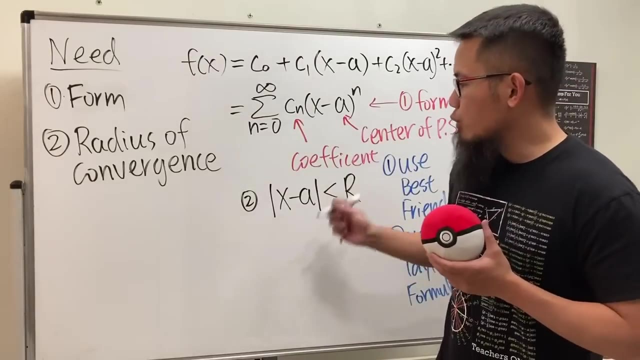 already you should. you should indicate that, okay, we have this, and then also notice that the second thing should write down the absolute value of x minus a to be less than r, and the r is precisely the radius of convergence. how do we find that? again, we can use the best friend, or maybe we have to. 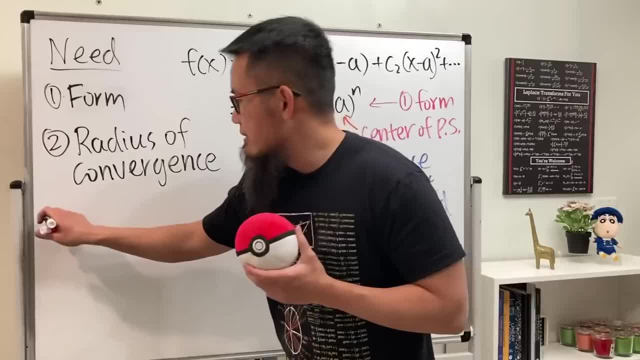 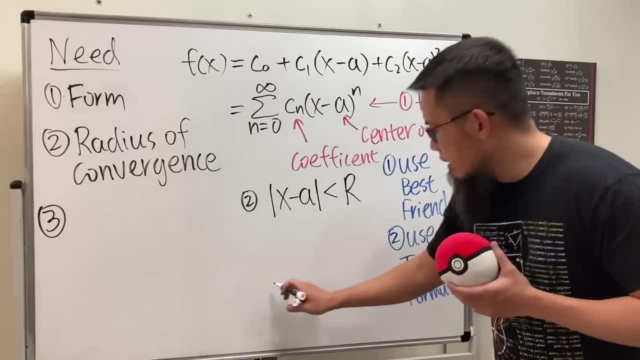 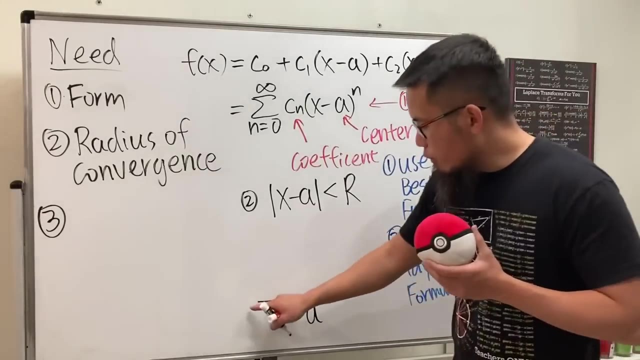 do something else, but that will be later on. the third thing is that, because when we have this inequality, we can open it. so this means what well we have the center, that's at a, and the radius in the one dimensional situation. it tells us that we can go to left and also the right r units. 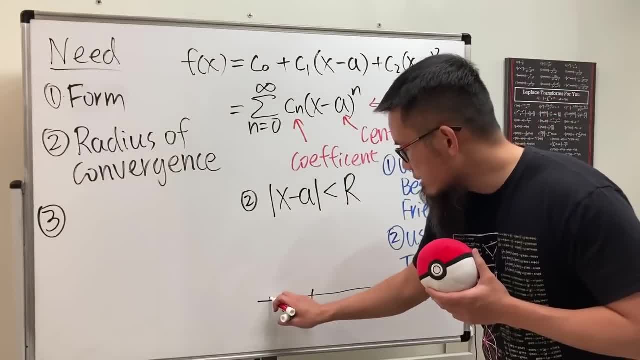 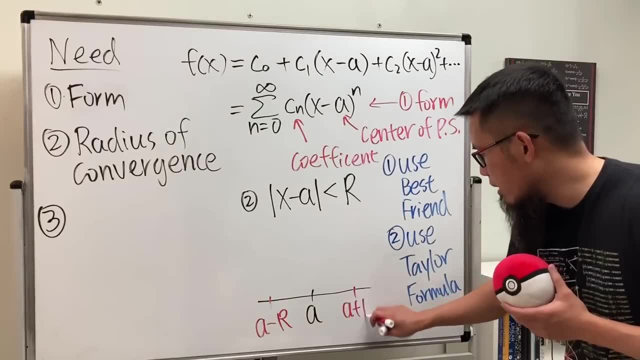 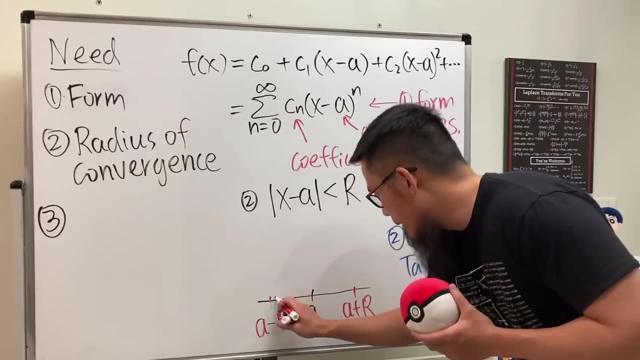 so right here, if we go to left r units, this right here becomes at a minus r. if we go to the right, at r units, we get a plus r. so, as you can see, we end up with the interval and the interval will tell you more information. so all the numbers inside of the interval: 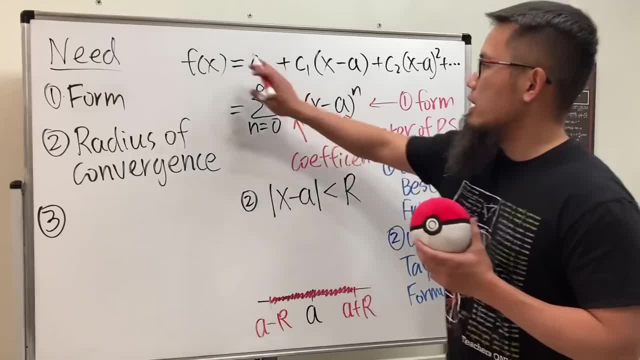 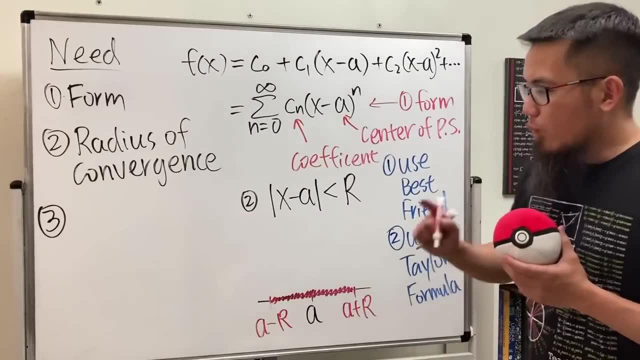 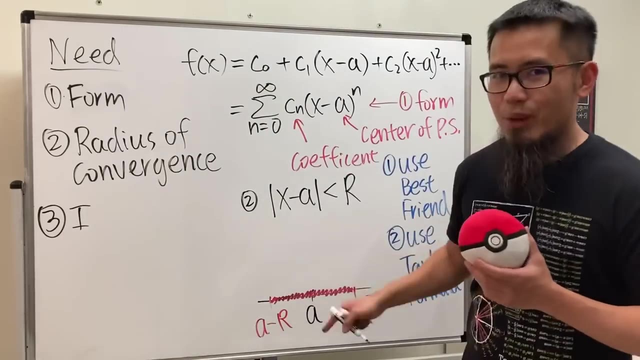 are the legitimate x values that can plug in into the power series and that will give you the correct function for the f. but there's one little problem with this right here, this interval first. let me write this down right here for you guys. first, this is called the interval. 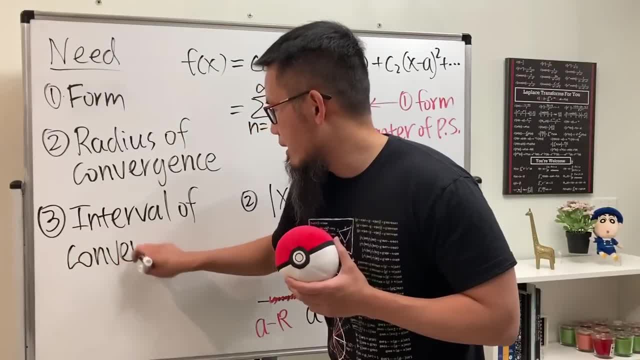 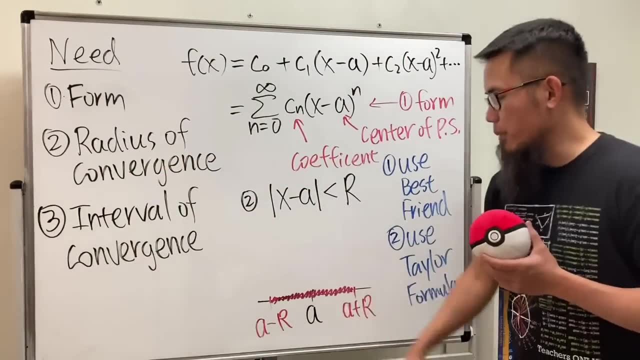 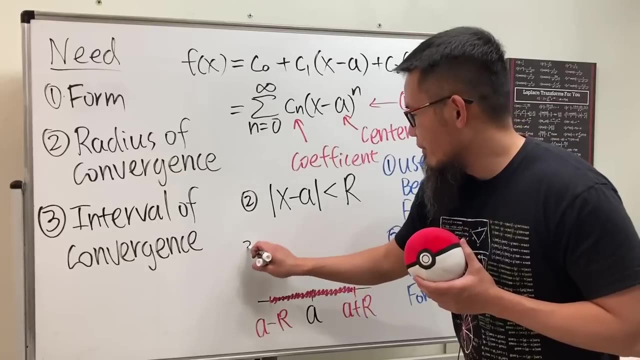 of convergence, and that's precisely the continuation of the second part. right, so once you have this, you should be able to get that. the trouble for this right here is the following: right, all right, let me write that down. when we see the picture, we can use interval notation for this and the notation 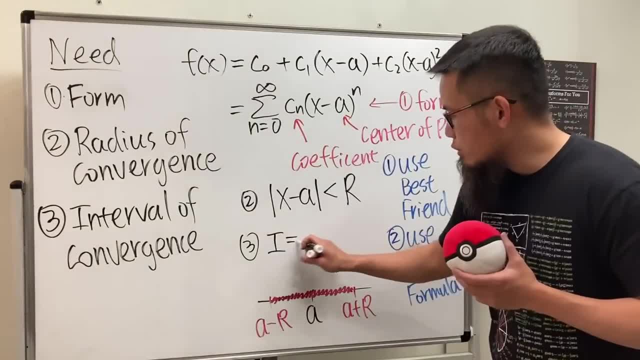 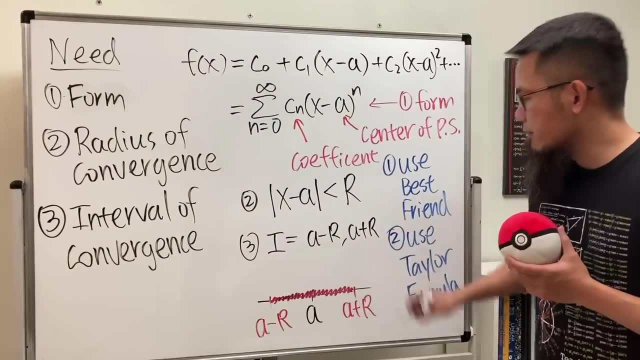 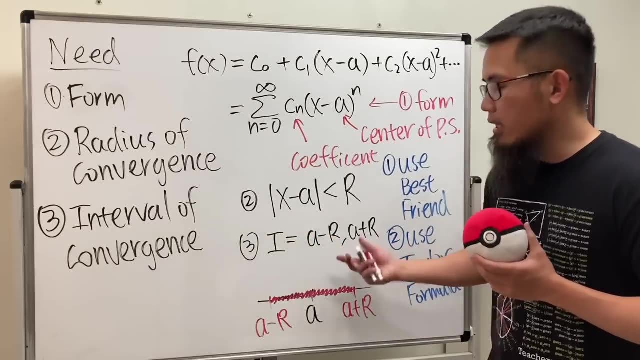 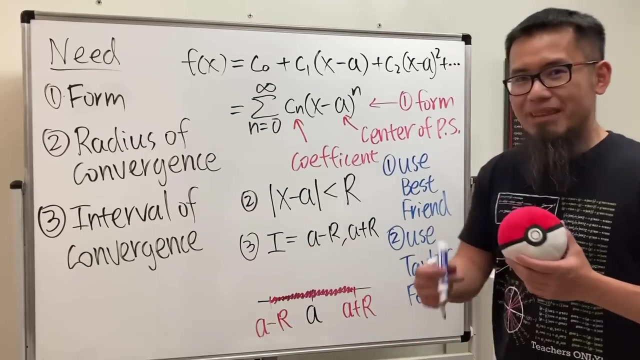 for the interval of convergence. just i, we have this right here become. it goes from a minus r to a plus r. but the trouble is, do i include the endpoints or do i not include endpoints? uh, parentheses with bracket. um well, let me show you guys this. have you guys seen this notation before? 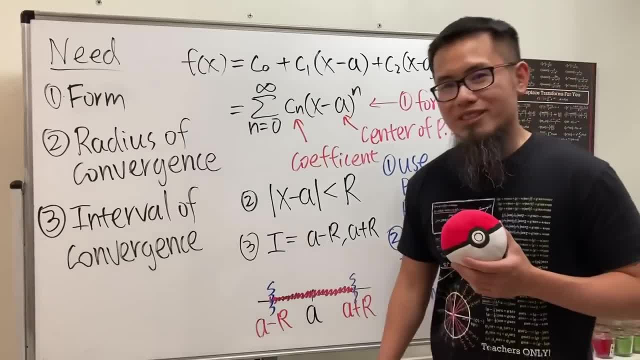 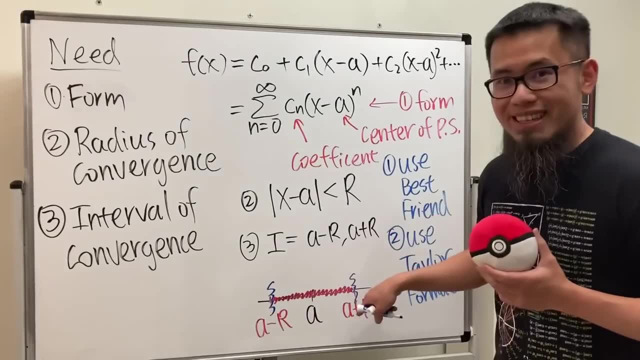 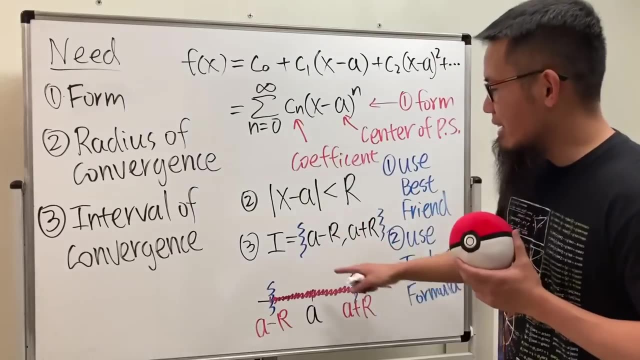 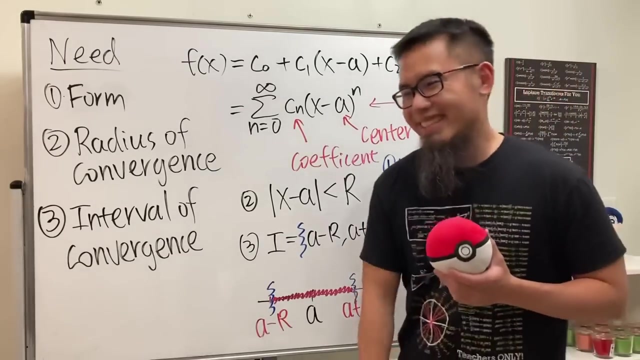 when you are working with interval notations. no, you should say no because i just make this up. so, and the reason is because we have no idea. we have no idea if we are going to include the endpoints or not, unless we do more work and do things. yes, we will have to do the 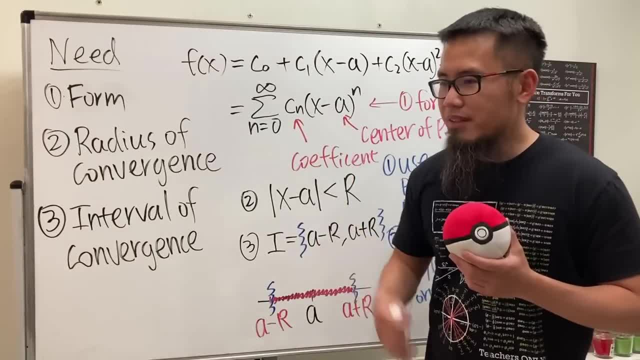 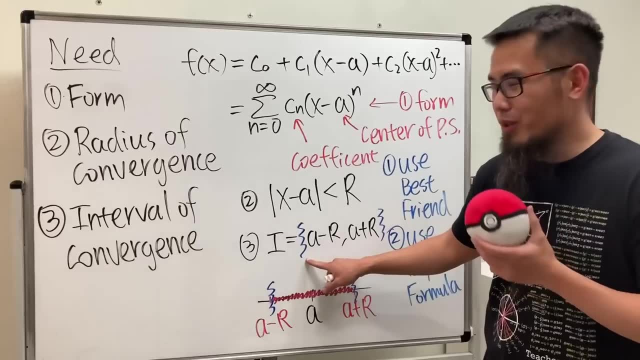 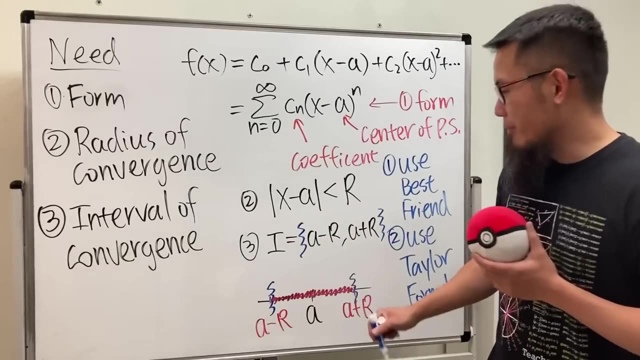 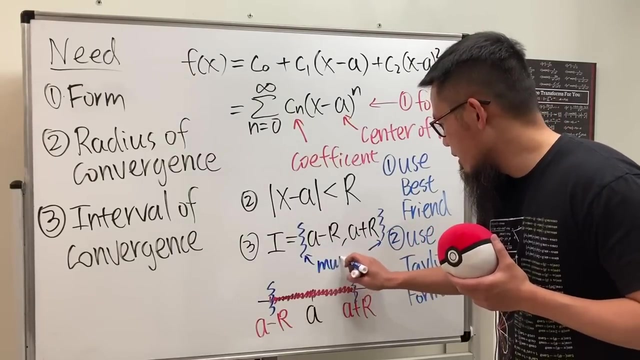 ratio test, direct comparison test, alternating series test, things like that. so all the series convergence tests are useful to check the convergence at the endpoints of the power series and for the interval. that yeah, so uh, i would just say must check, must check with the convergence tenses. 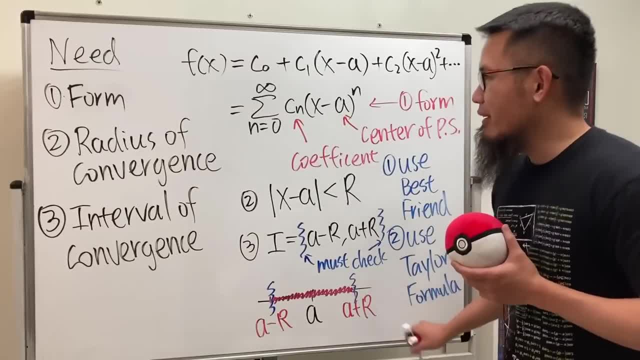 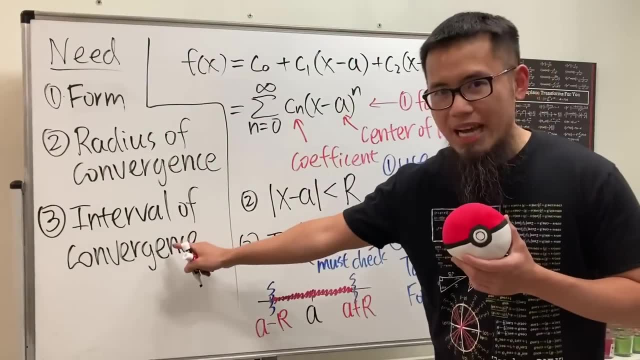 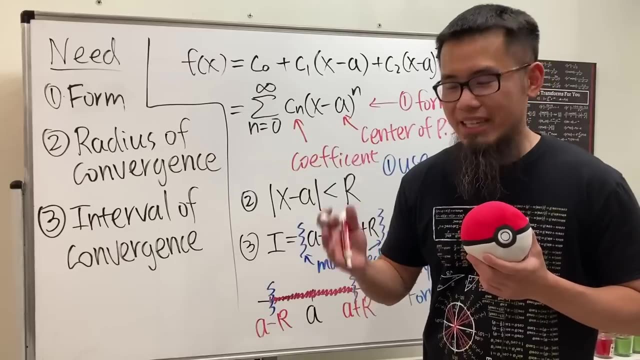 yeah. so this right here. just keep this in mind- we have the three things that we need: the form, the r and also the i. but today we are going to finish this happily, because we will look at the best brand right now. so we'll start with the geometry series right here. 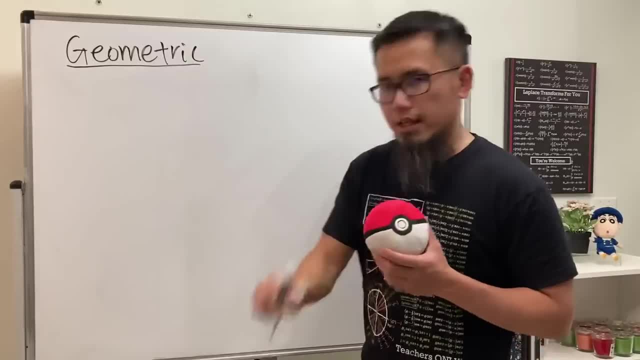 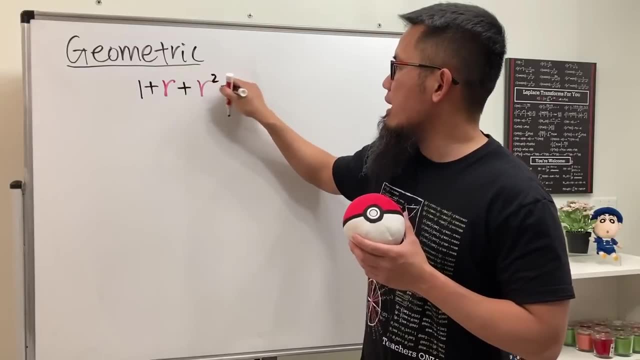 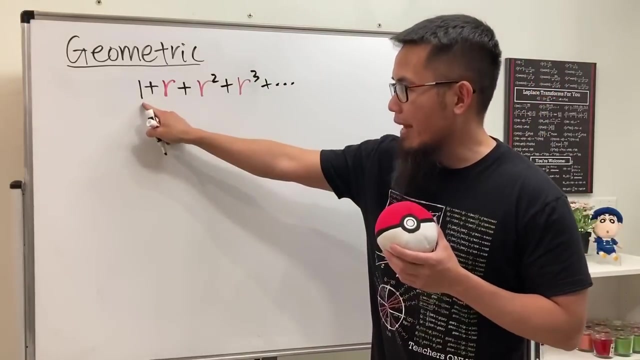 and this is the one that we are going to be looking at, starting with one, and then we are going to add it with r, and then r square, and then r to the third power, and then so on, so on, so on. well, we know that the first term is one, and then the common ratio is r. if this is nice enough, then 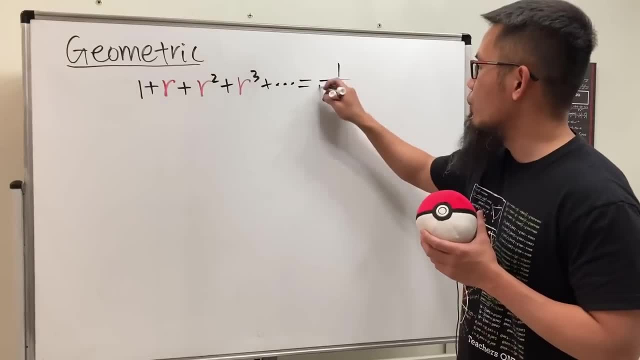 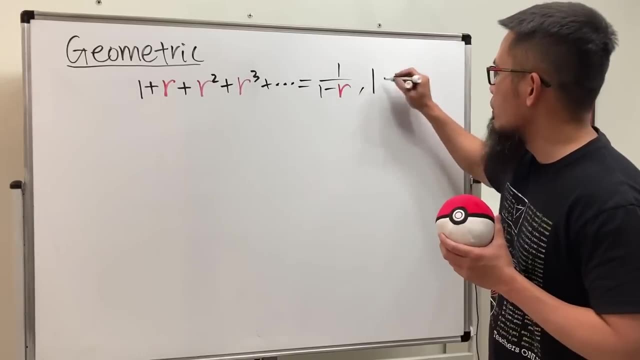 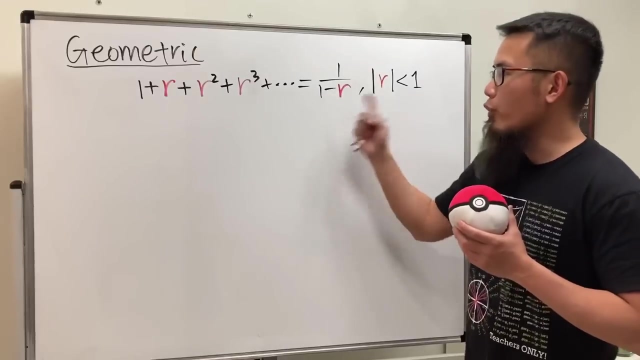 this right here will converge to the first term over one minus the common ratio. right, and we know this right here is nice enough when the absolute value of r is less than one. if this happens, then this right here will converge to one over one minus r, which is very nice as we can see the left. 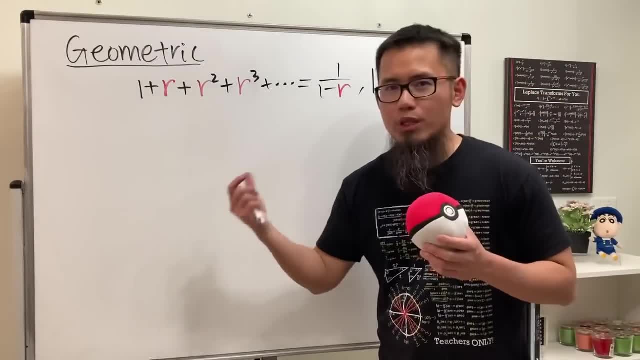 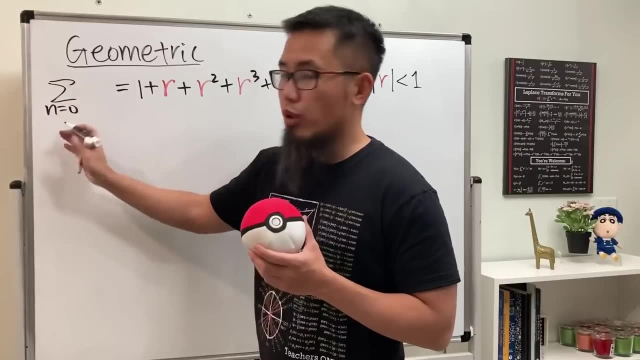 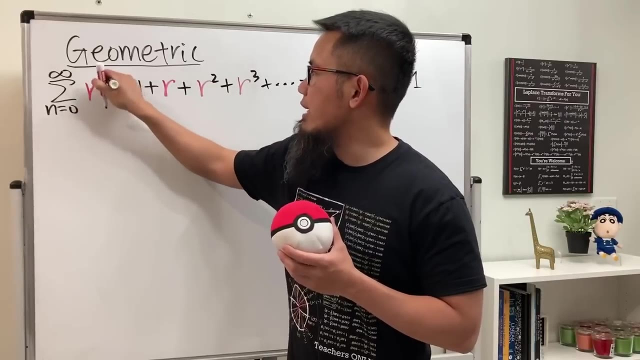 hand side is the expanded version. of course we can put that down into the sigma notation form. so it becomes the series. so it becomes the series as n. let's use zero right here, and then infinity, because n start with zero. we can just write this down as r to the nth power, just like that. very nice now take a look right here. earlier we put 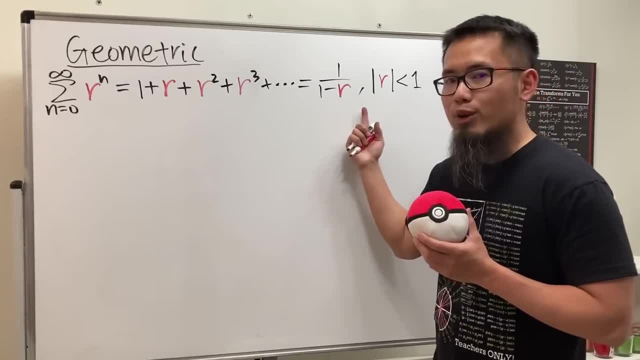 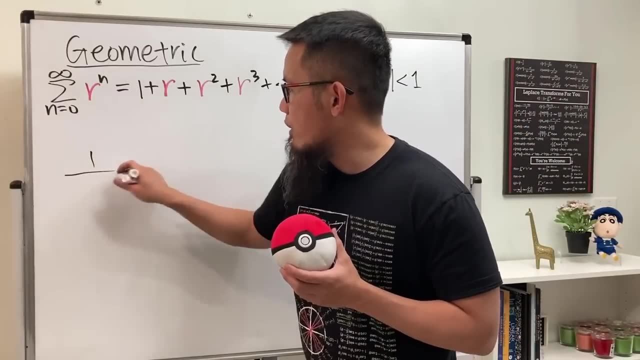 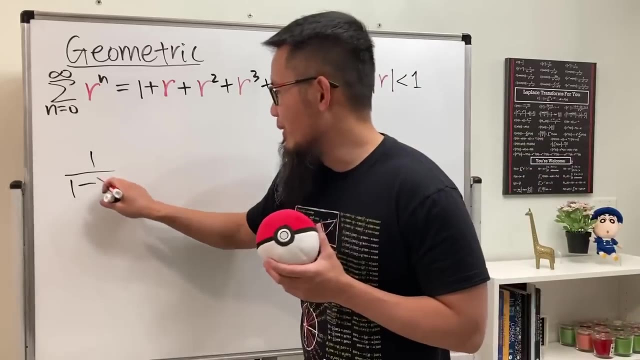 this down from left to right. right now we are going to look at this backwards, so i'm going to put this down first. so let me write down 1 over, 1 minus. but instead of using r, i would like to use x, so we can look at this as a function, and now all we have to do is replace. 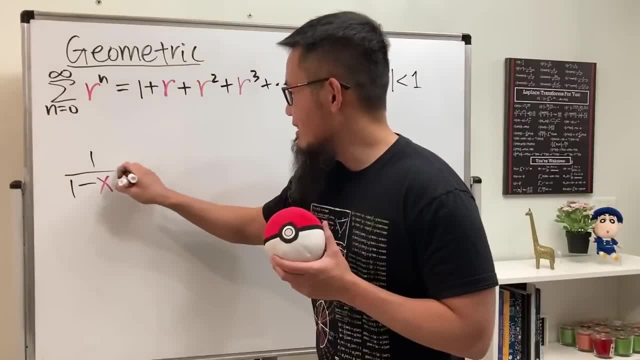 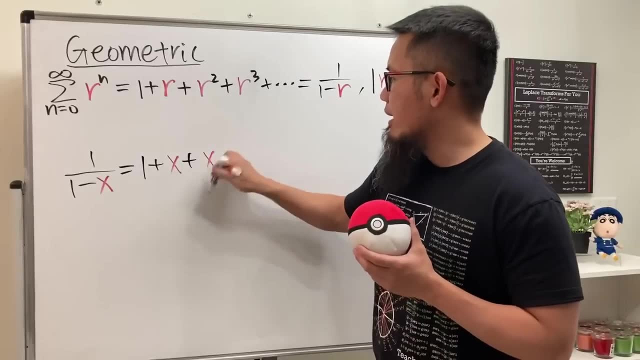 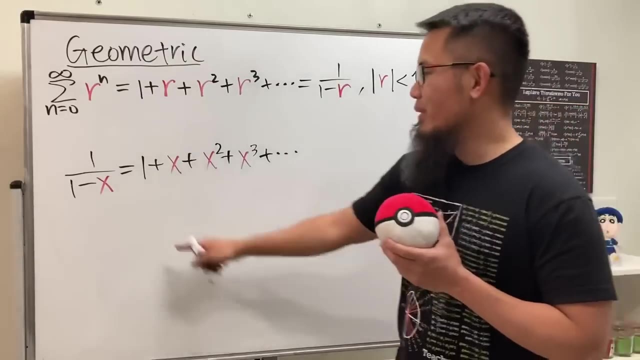 all the r's with x's, so we can see that this, right here, is equal to 1 plus x plus x square, and then x to the third power, and then so on, so on, so on, isn't it? and of course we can also put the x right here so we can get what? yes, the series as n goes from zero to infinity and the derivative is cancels out. So we need a octopus. 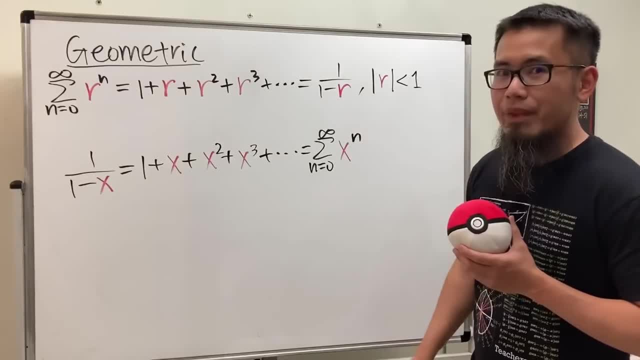 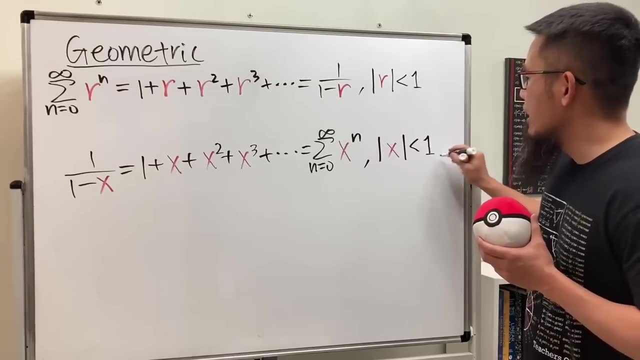 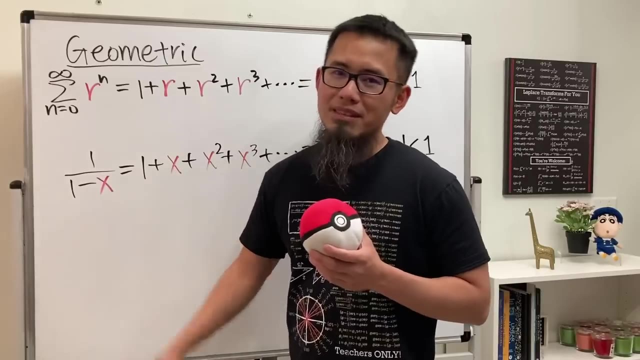 infinity x to the nth power, and we can also write this down as: the absolute value of x has to be less than 1 in order for this to be legitimate. as you can see, this is the function 1 over 1 minus x. it's a rational function. this is the expanded version of the power series. 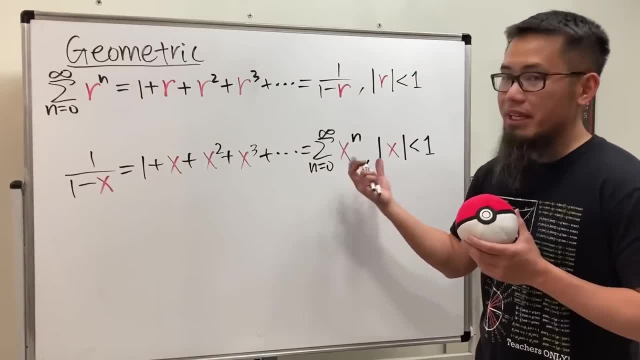 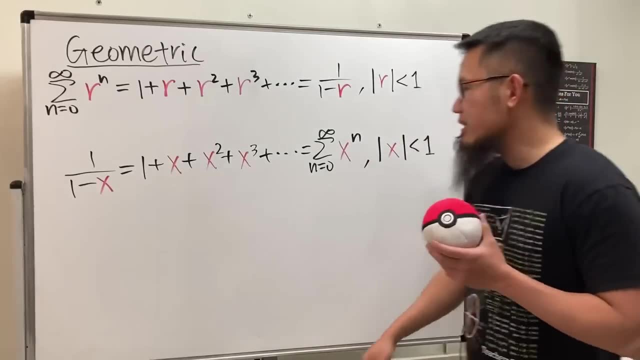 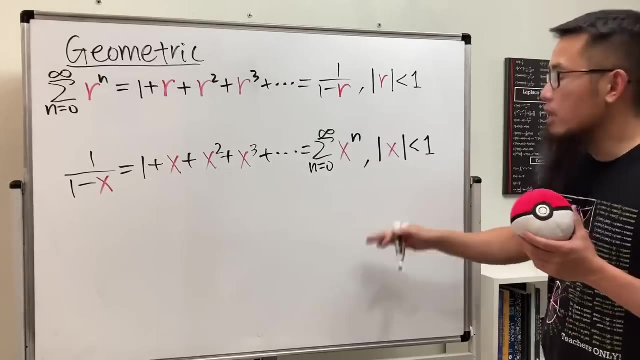 and then we have also the power series in the sigma notation, and this is exactly the form that we need. so we have the first thing, and the second thing is that, based on this, you can see well, because it's x only, it's not x minus 4. so this right here tells us: the center is at 0. 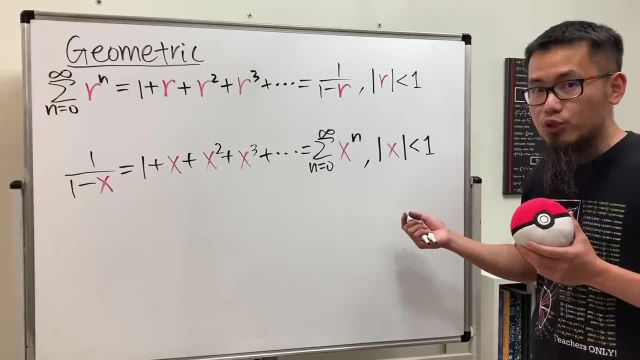 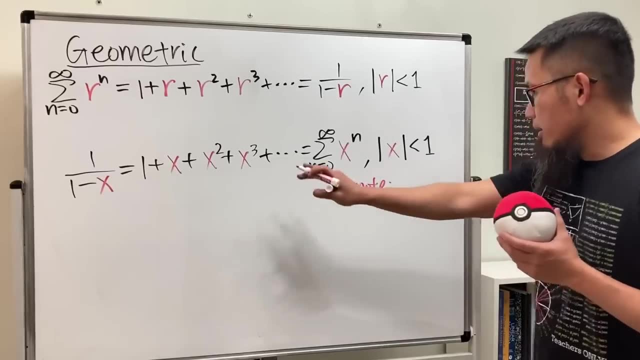 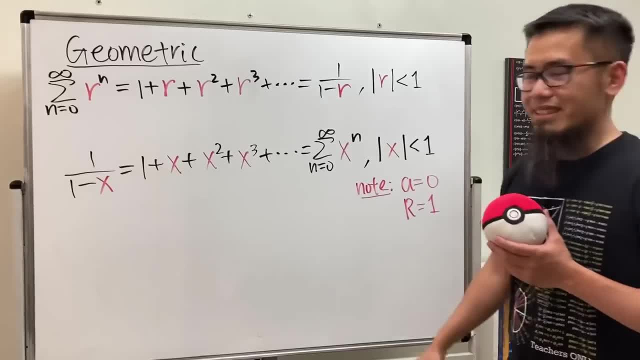 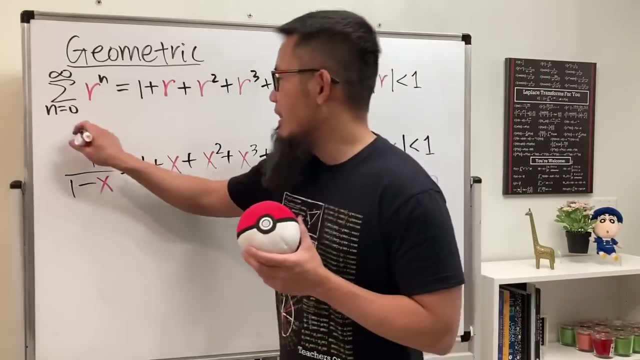 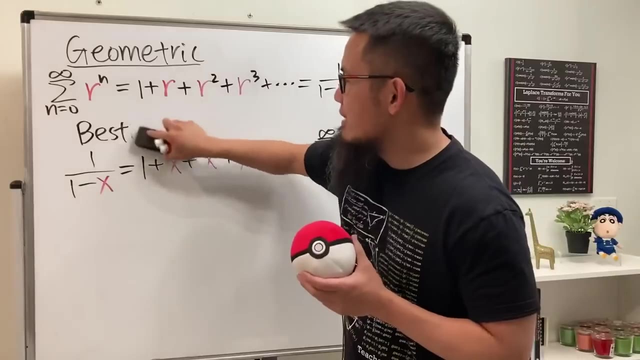 y is equal to 1. so nice, isn't it all. right now, this, right here, is exactly what i call the best friend, and nowadays you can also call this to be the bestie, because i think this is the popular word nowadays, especially on tiktok. but i've been calling this the best friend for about like five. 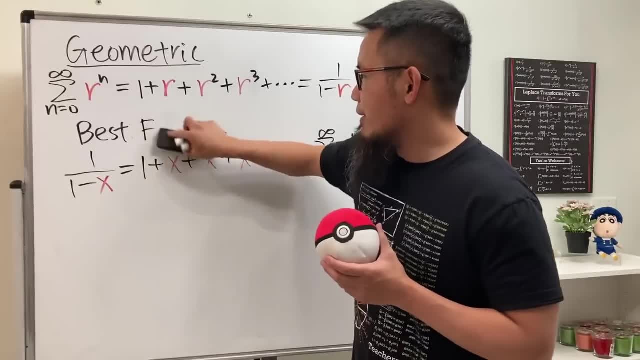 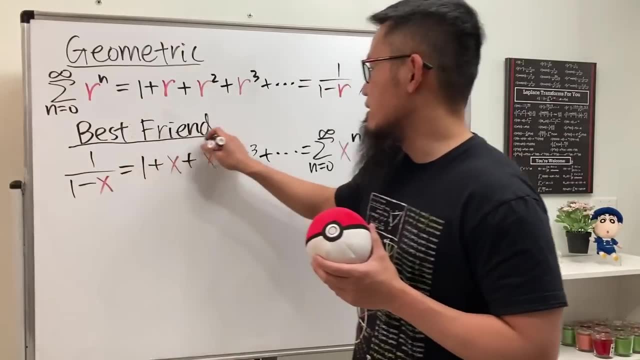 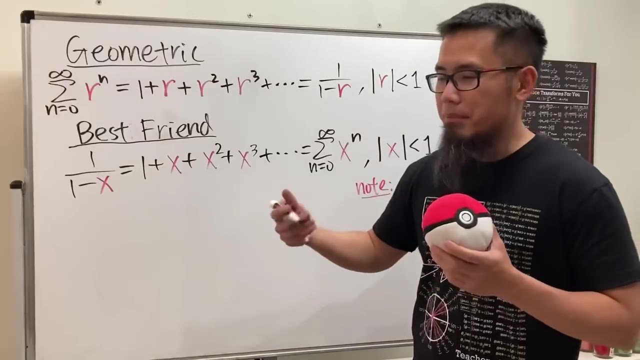 six years already. so i will you know, keep writing it down, best friend, like so, and i would really like to show you, guys, why this is the best friend. hopefully, after all this, you may also want to call this the bad, the bff. best friend forever, anyway, though. 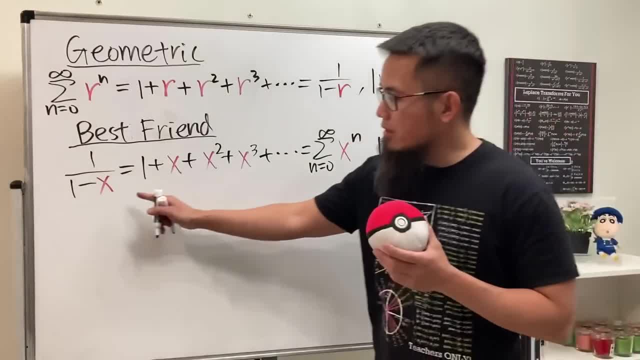 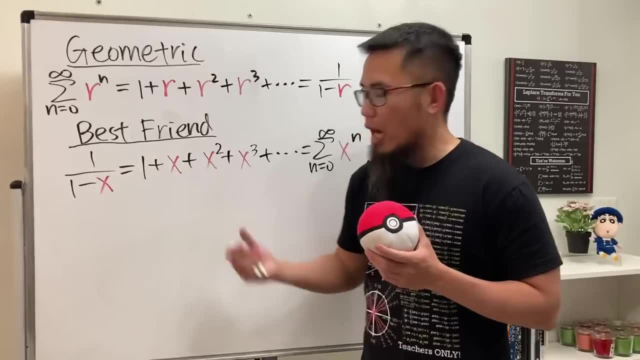 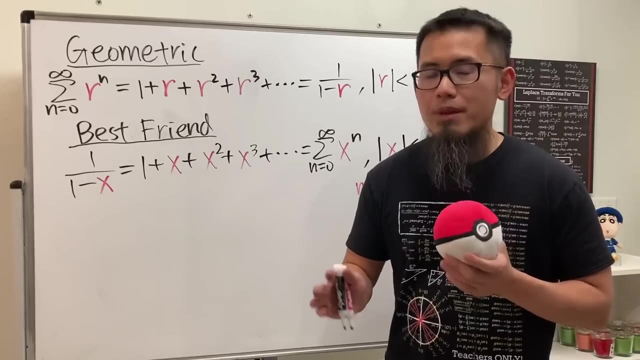 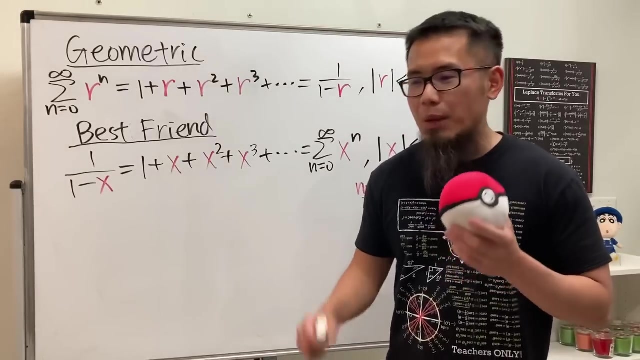 one reason that this is the best friend is because, you see, we actually have the power series already, but it will also help us to get more power series of more functions. in fact, i have a video called the power series marathon where i have done 26.2 power series for you guys already. i will link. 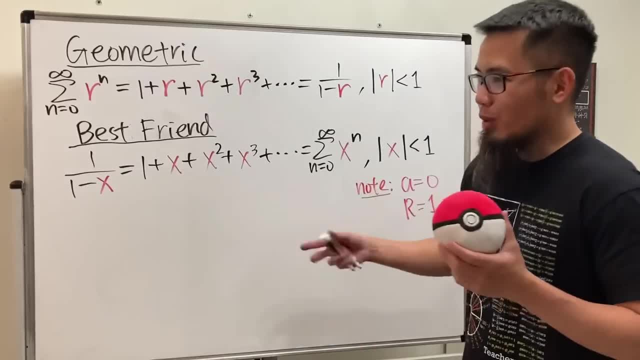 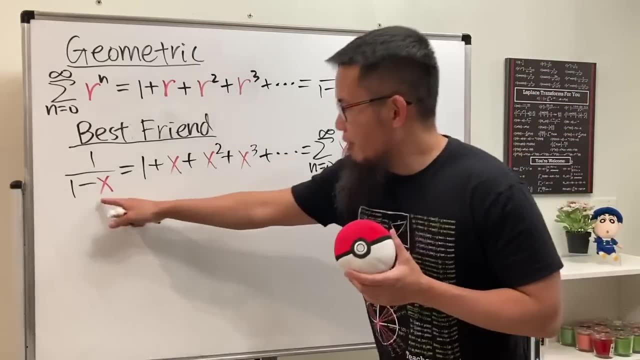 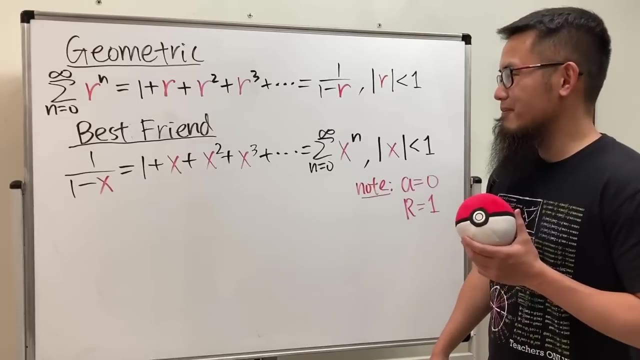 that in the description, for your convenience. so i'm not going to work out all 26 again, because this video is just trying to introduce you, guys, the concept power series. this is the first one. ladies and gentlemen, have a look, right, have a look. so nice isn't it? and 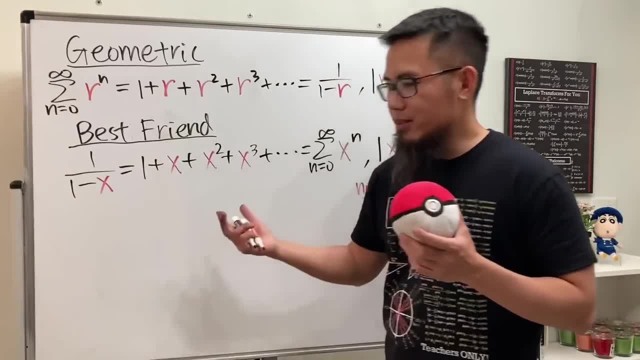 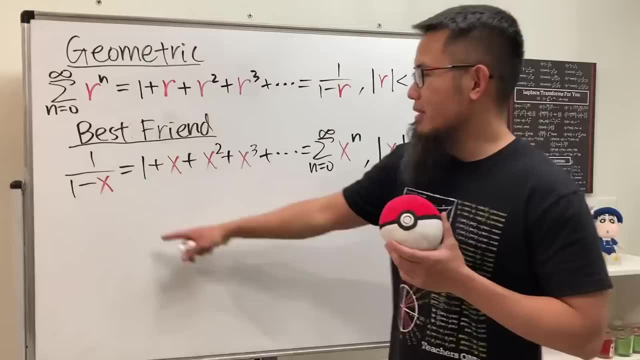 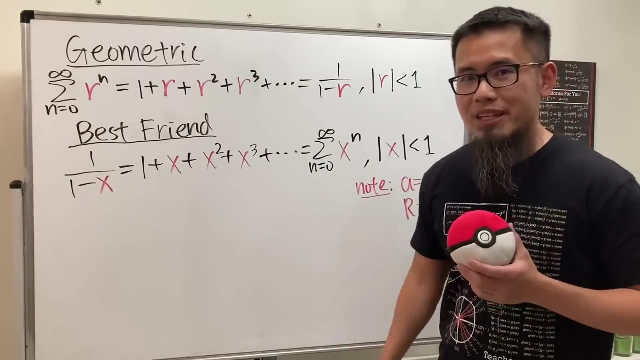 you know, i like to just assign things names, so that way we have some like, um, better feeling about the questions, better feeling about the math, because, okay, here's the deal. if i just call this the geometry series, ah, people will be like, no, i don't want to learn it. but if 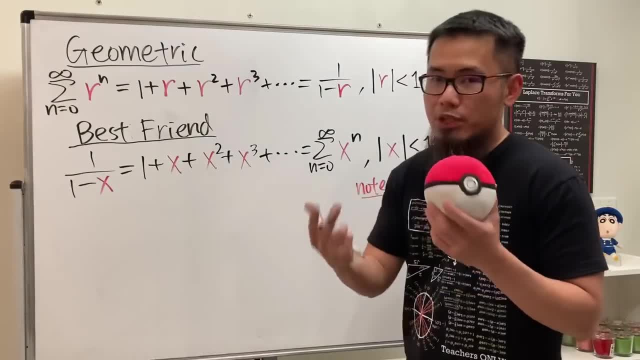 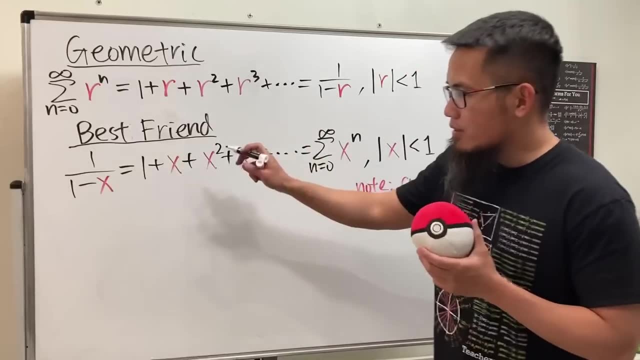 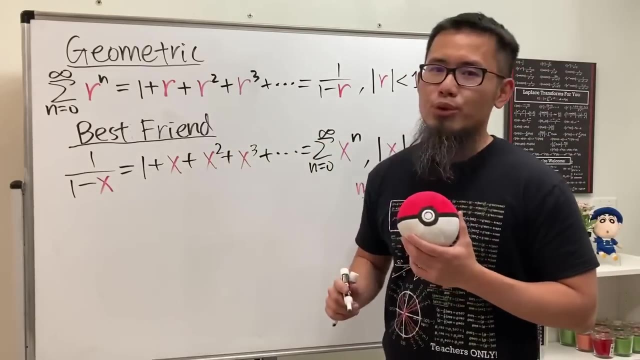 i call this the best spread, which is actually really beneficial, because he actually helped you to do a lot more. best friend- who doesn't like best friends? right, and of course, when we have a best, we need to know how to use it. i know it sounds so bad, but in math it's totally okay. anyway, though, 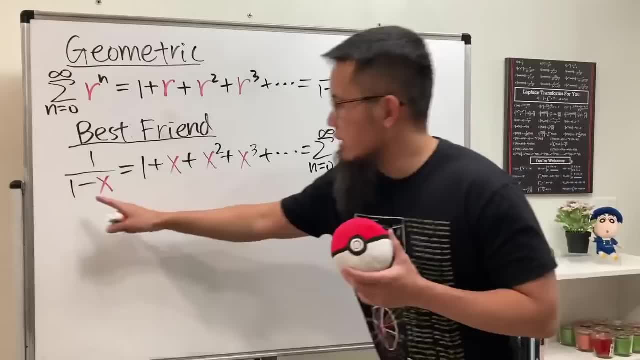 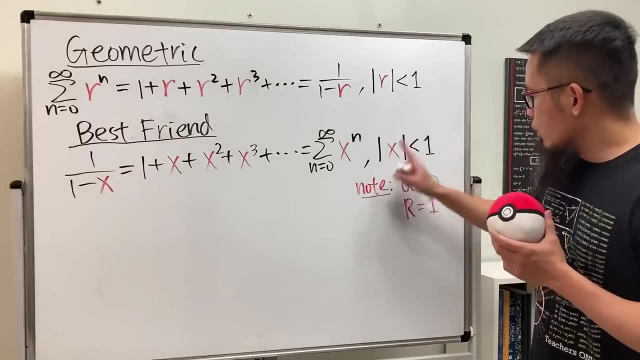 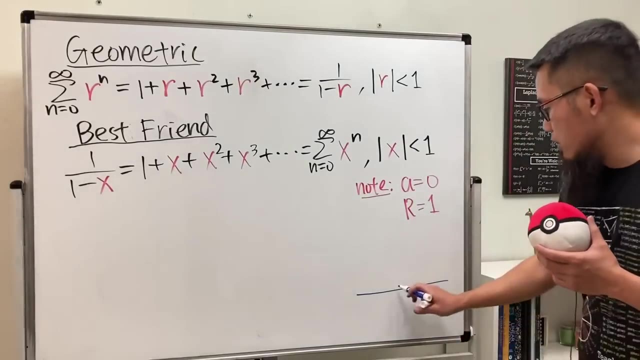 i would like to explain to you guys this function and this right here, and also what the r represents. and, by the way, we have this already, so we can draw the interval of convergence. the center is at zero and then, you see, the r is one, so we can just go to the left one unit. 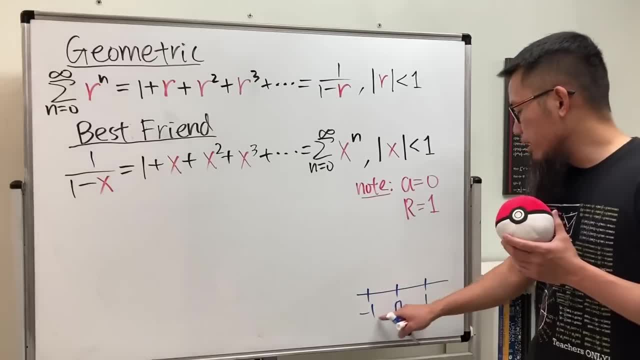 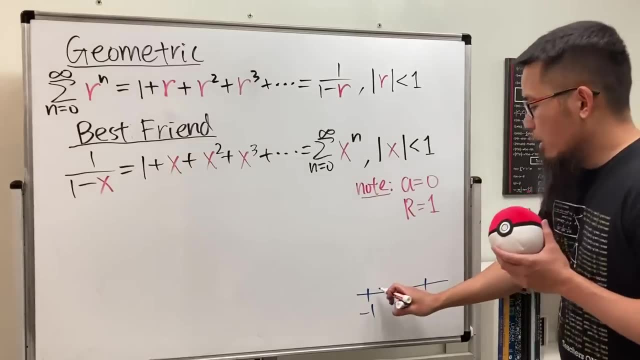 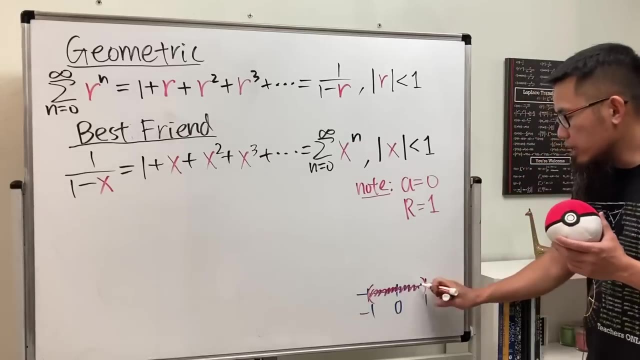 and then go to the right one unit, so we go from negative one to one. and for the best friend right here, i would like to tell you we do not include the endpoints, so you can just keep that in mind why. one way to do it is you just put a one in here, then just get one plus one plus one plus one. 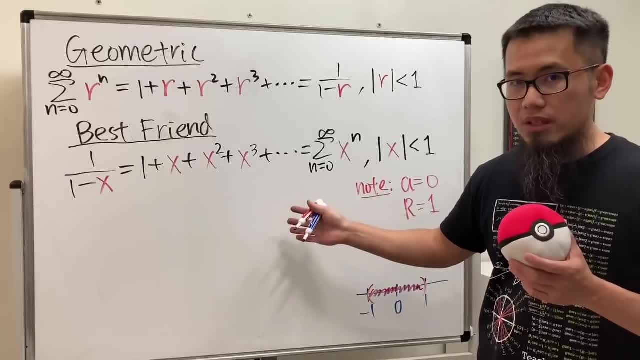 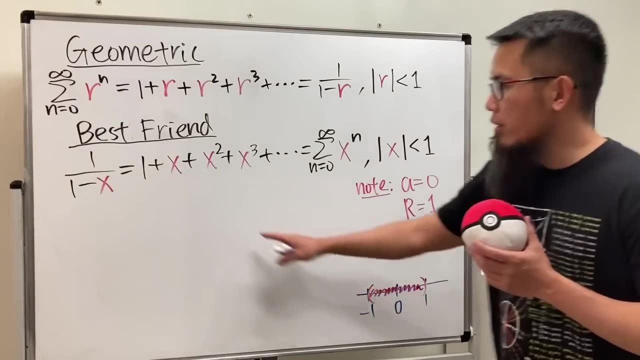 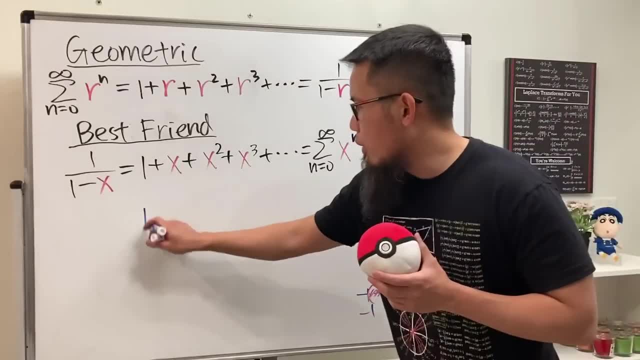 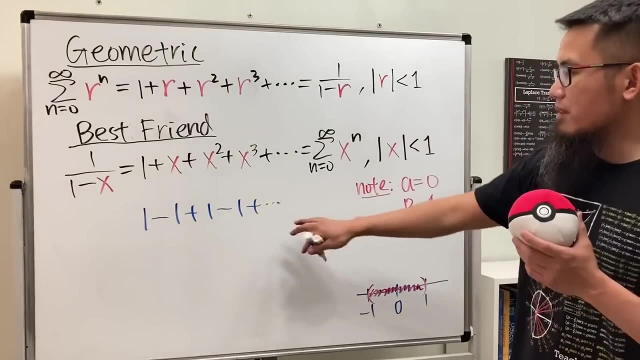 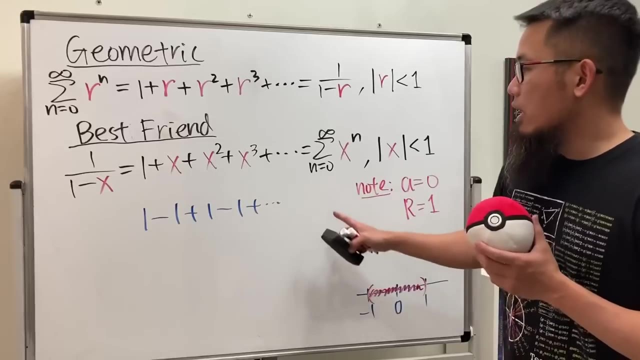 situation you actually get when you put negative one, you get one minus one plus one minus one, and then you get a weird sum right, you get a weird series. it does not converge. one simple reason to say this does not converge is because, remember, for the geometric series, the absolute, 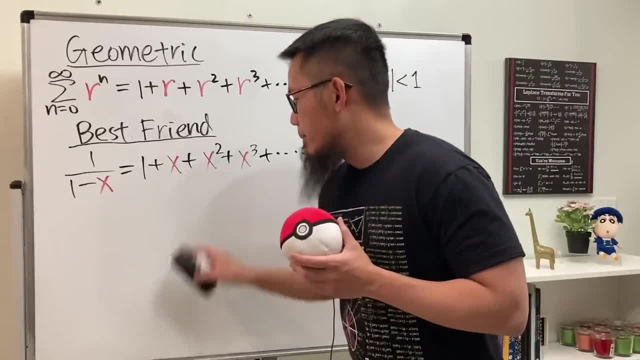 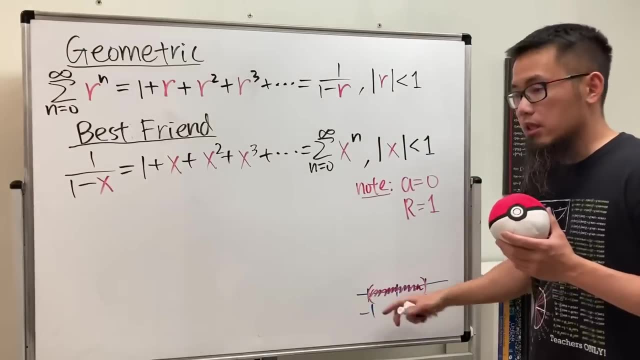 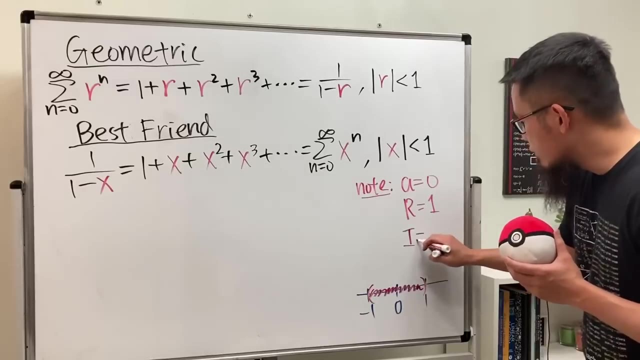 for your r has to be less than one. but later on be really careful with this notation when we do the other power series, because we really have to check the endpoints right. the convergence at the endpoints for the best spread, i can tell you the i goes from negative one to one and we do not. 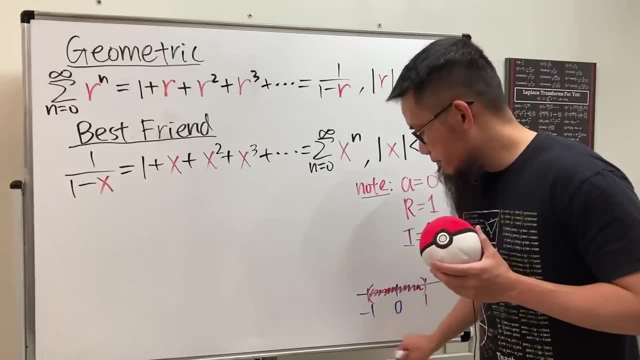 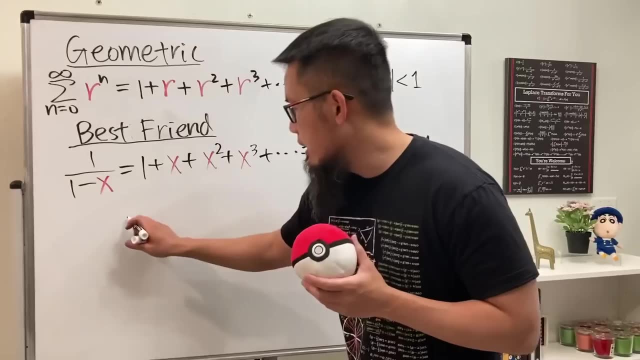 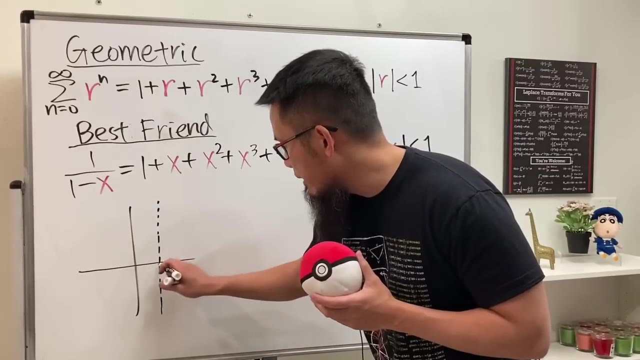 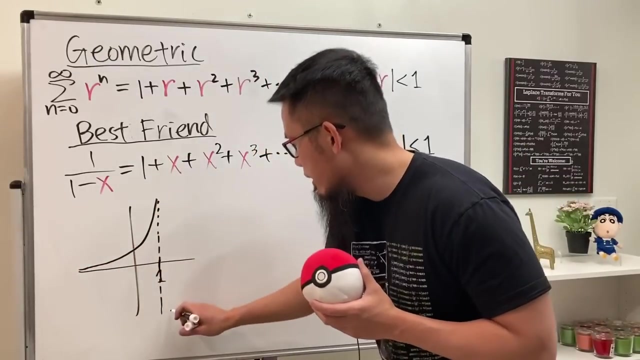 include the endpoints, right? so that's that. now take a look at the graph of one over one minus x, which is just a rational function and it has a vertical asymptote at one. so let's say: is right here, this is at one, and the graph of that looks like this: go up like so and then go up like so. all right, 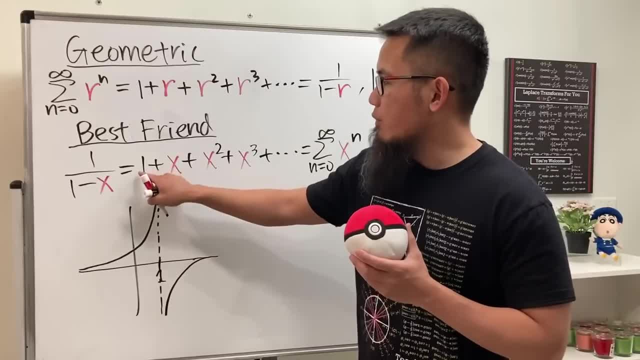 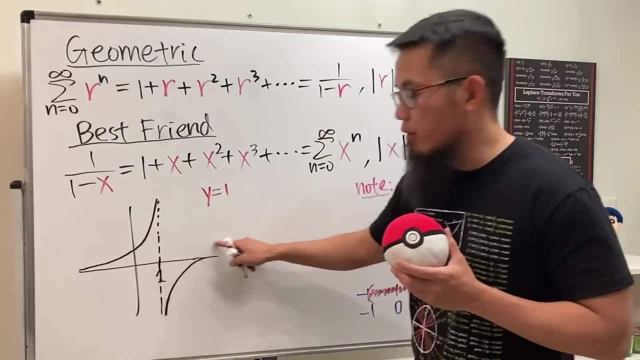 now take a look at this. we have one for the first term and if you just make a graph, y is equal to one. that's just going to give us a horizontal line right here and you will see the horizontal line cross the curve right here. that's it pretty boring. 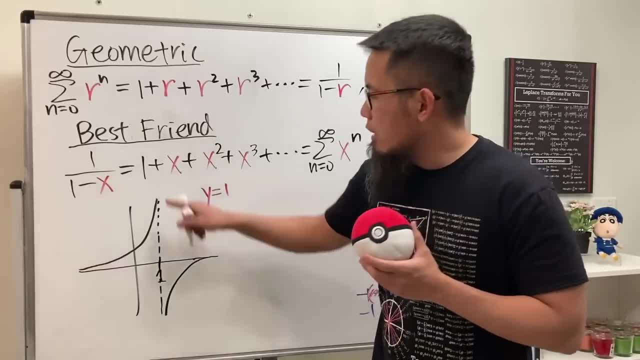 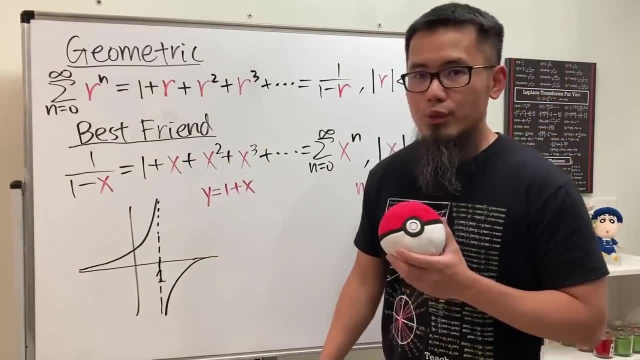 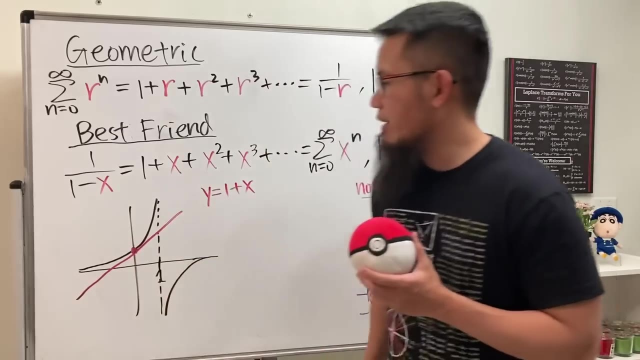 because they only intercept at one point. if you include the next term, which is now one plus x, if you grab this right here, you get what you get a tangent line right here, and that's the calculus term for that. you get a line tangent to the curve. 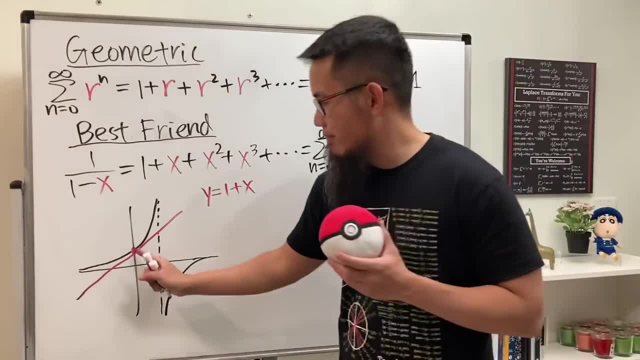 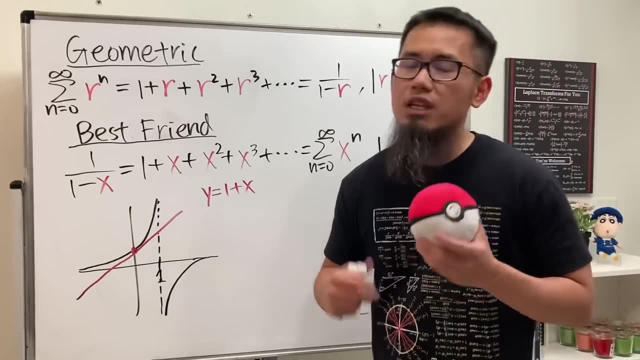 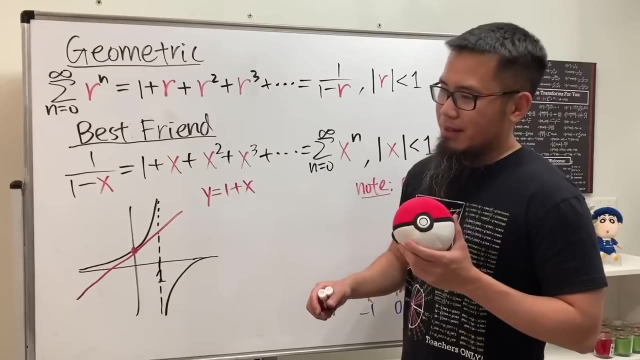 at x equal to zero. x equal to zero. that's exactly the center right here. could you have different centers? yes, but you will have to change the form of the power series, and again, you will have to watch the power series marathon to find out how to do it. anyway, though, as you can see this right, 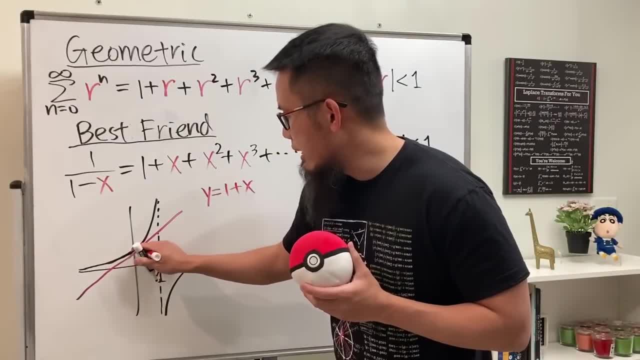 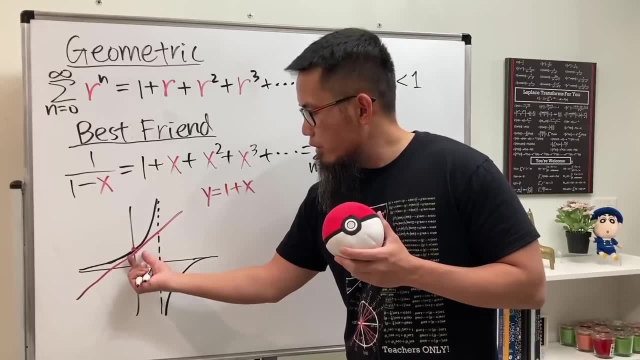 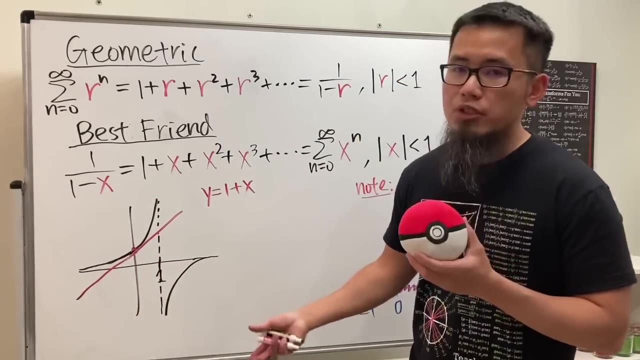 here is the curve and this right here is the tangent line and if you look at the line and the curve, they are pretty close to each other around this region right here, right, okay, and that's the cal, one way to approximate a curve, the linear approximation, right, locally speaking. 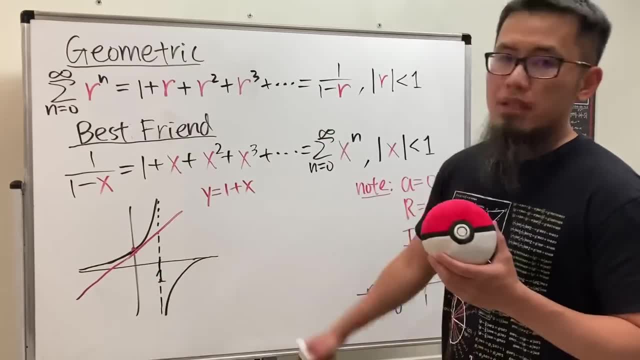 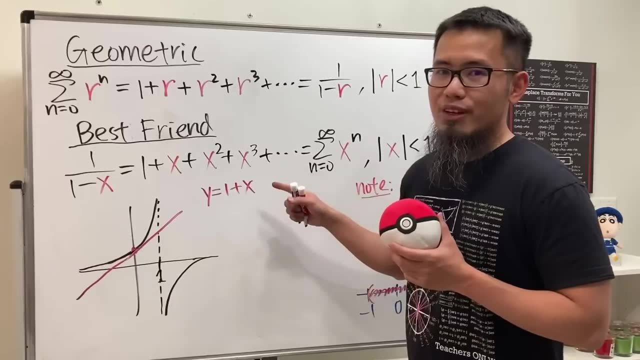 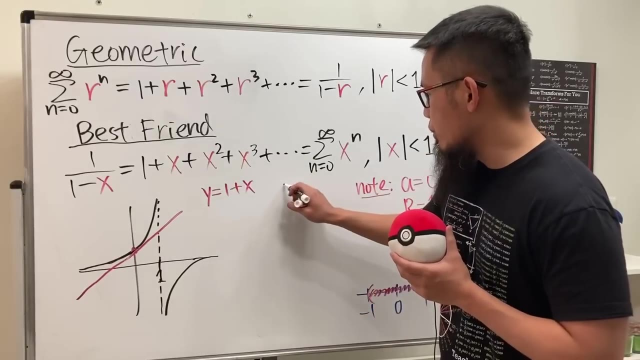 can we do better? of course, because we're in cal two now and to do so, you know what? we have a lot more terms right here. all we have to do is just keep putting more and more terms, and let me show you guys another picture right here, real quick. 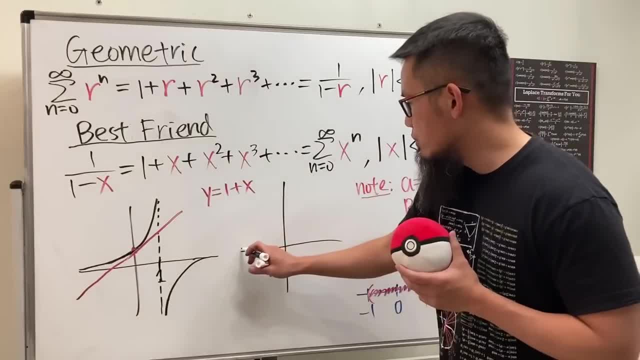 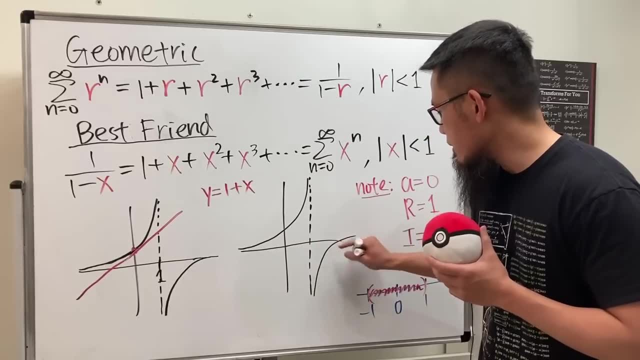 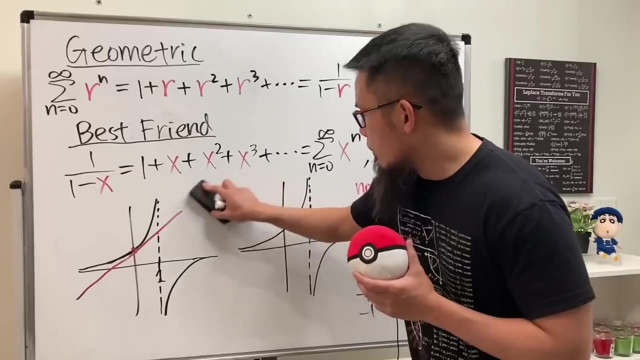 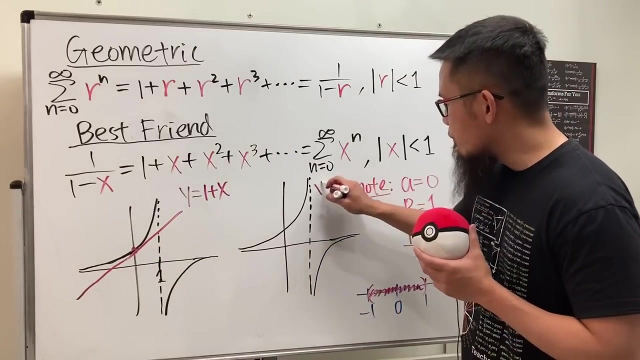 suppose we do the picture again which is one over one minus x, and then again we have the vertical asymptote and then we have this right here. bad picture, i'm sorry, but yeah, you get the idea. okay, well, earlier we have this right. y is equal to one plus x. now, if i want to grab, y is equal to. 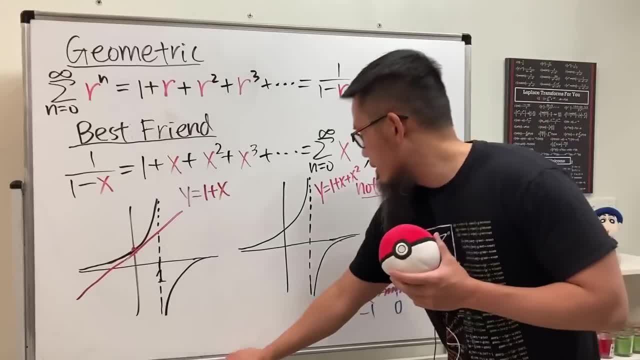 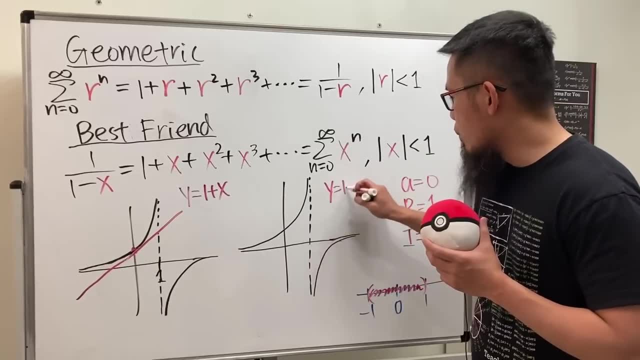 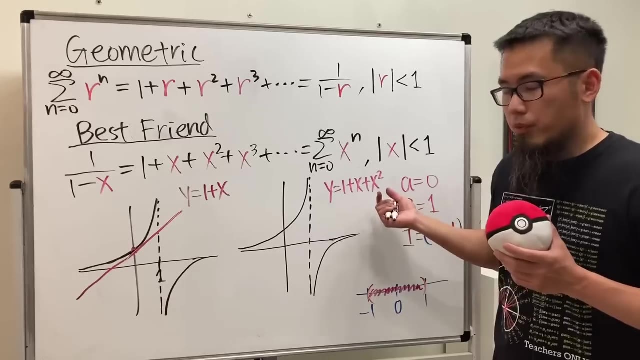 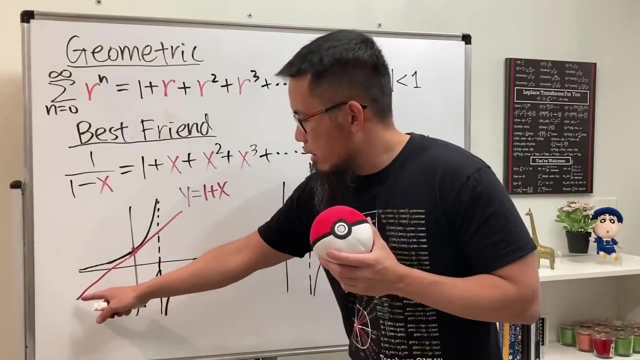 one plus x plus x squared. so let me just write that down here: y is equal to one plus x. and then we want to add one more term, which is x squared. so what does this do? well, you can think about the following: the center is like your starting point, the approximation. 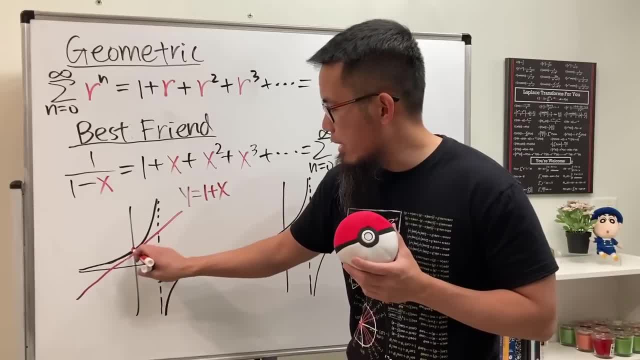 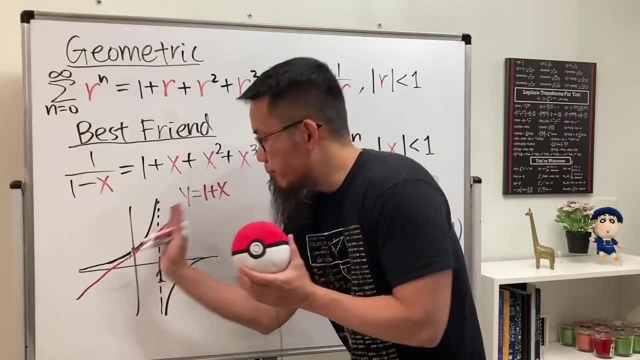 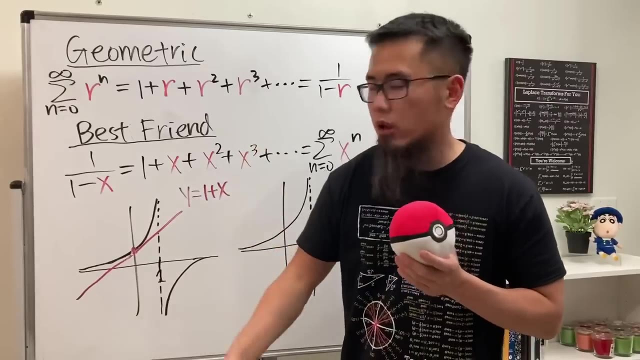 like the line right here, will touch the curve right here at this point. all right, and then, after you add more and more terms, what you are doing is that you are going to be able to get the uncertainty because you are going to be able to walk the curve right here. okay, so we are going to 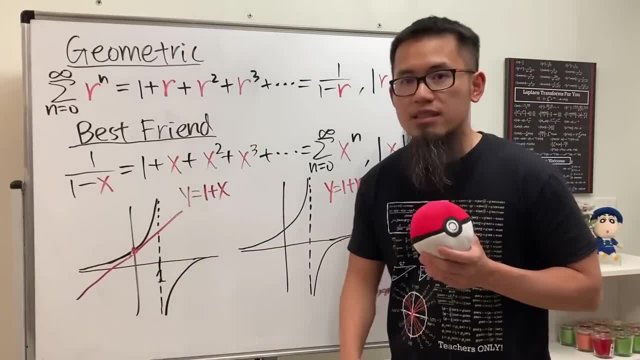 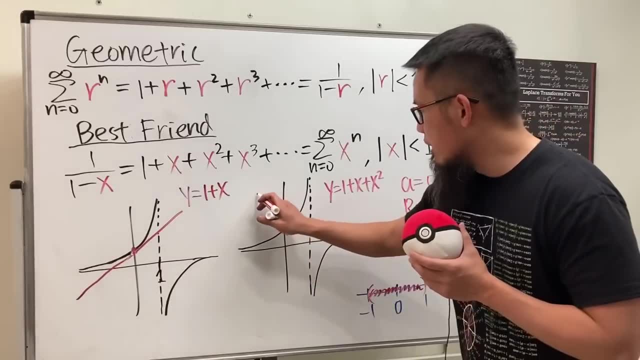 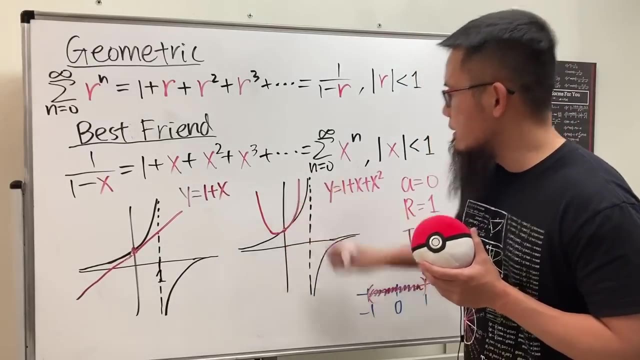 pass this point over, and so what you are doing is that you are going to bend the line and then, over and over, and, over and over again, just start going to bend the line. you're going to bend the line so that the red will become more and more like the black curve. that's the idea, and if you 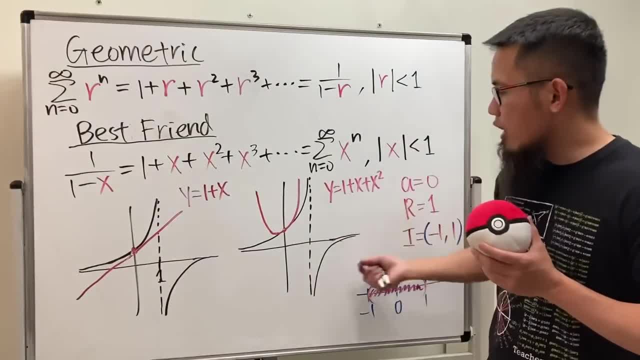 graph thislet me tell you: you have this and just bend up and you will get a parabola, because it's a second degree polynomial here, and you will get like this right and, as you can see, when you have more and more terms, then if you easy turn and you all have three or four turns, you will You. 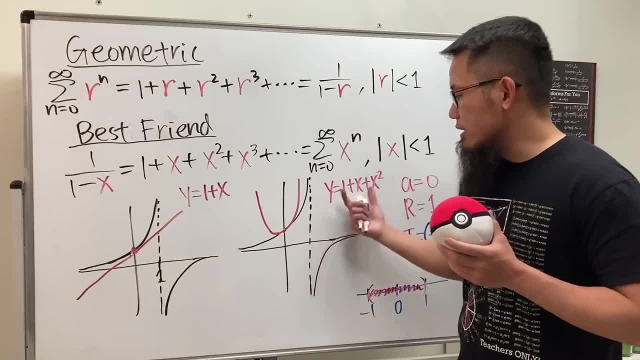 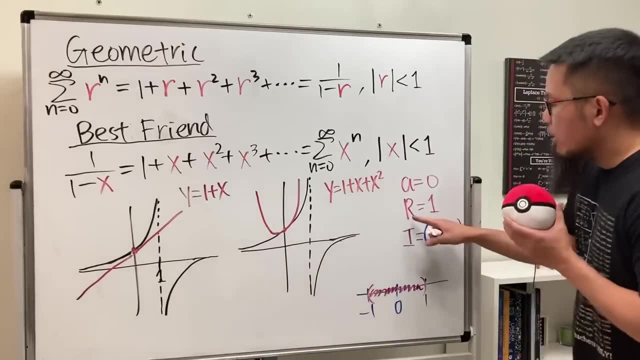 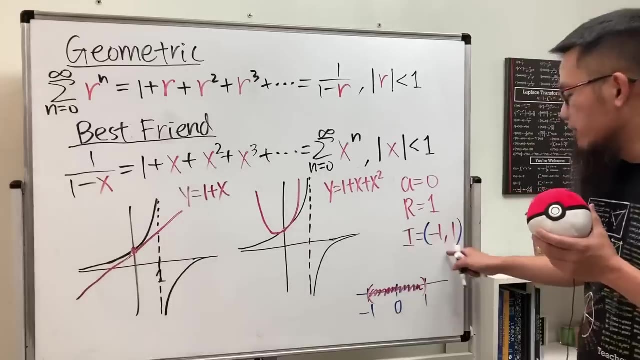 you will be able to approximate the curve with this polynomial: better and better. that's the idea. one thing to notice is that, though, when you have the radius of convergence, if this is equal to what, well, you can also look at the interval convergence. either way, you will be looking at from negative 1. 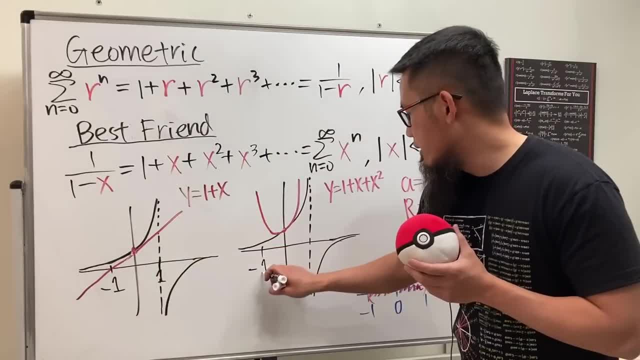 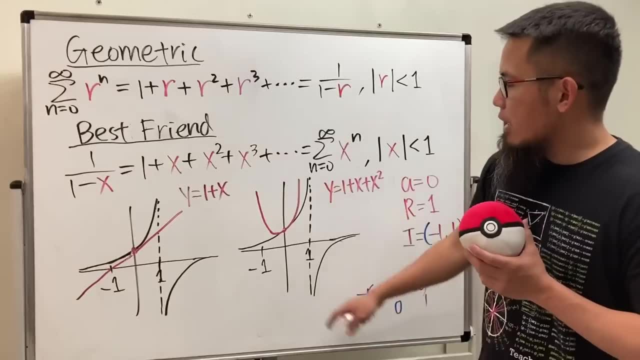 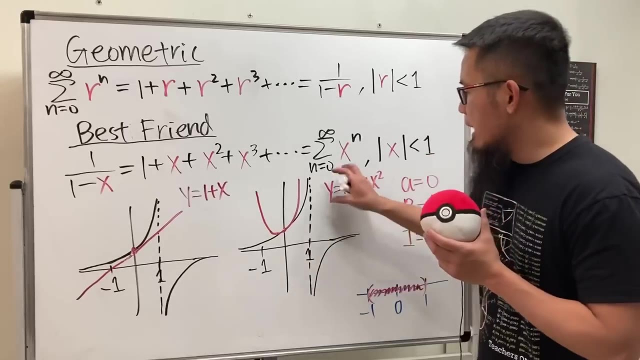 to positive 1, right negative 1 to positive 1. let me tell you, though, unfortunately, for the best spread, no matter how many terms that you add, if you have infinitely many terms, the best thing that we can do is that this red curve is going to be like this: only covering this part. you can never. 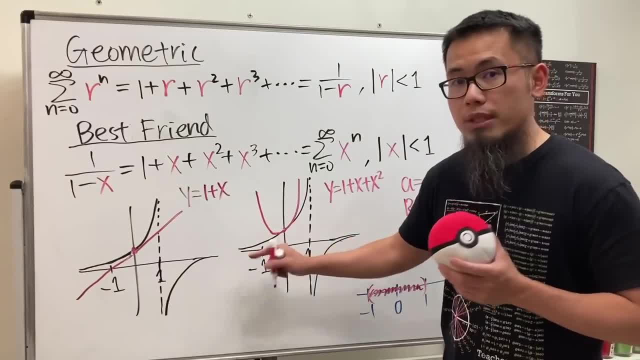 use this curve and touch this point because this point is outside of the interval convergence. you can never use this curve and touch this point because this point is outside of the interval convergence. you can never use this curve and touch this point because this point is outside of the interval convergence. 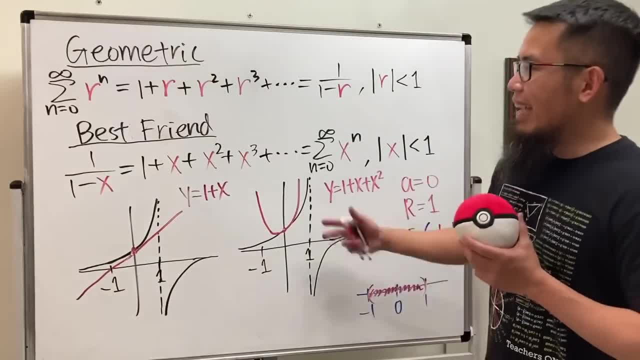 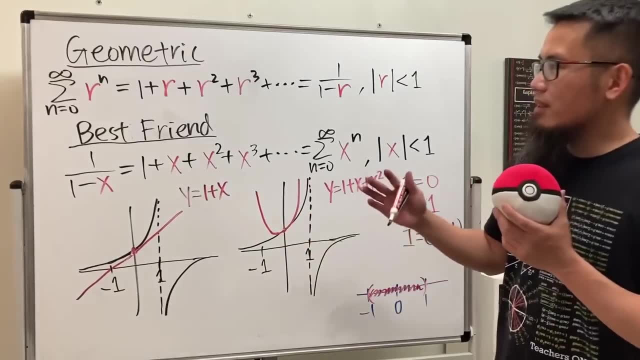 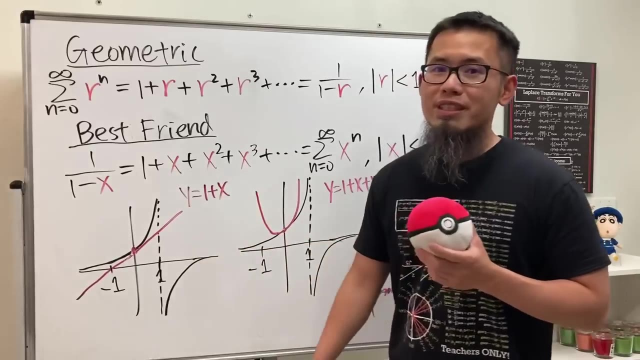 unfortunately. so that's the idea and i think this is enough for this video. hopefully, you guys all have a better understanding regarding what power series is all about and you have a better understanding with the purpose of the power series. seriously, it's just like having the decimal. 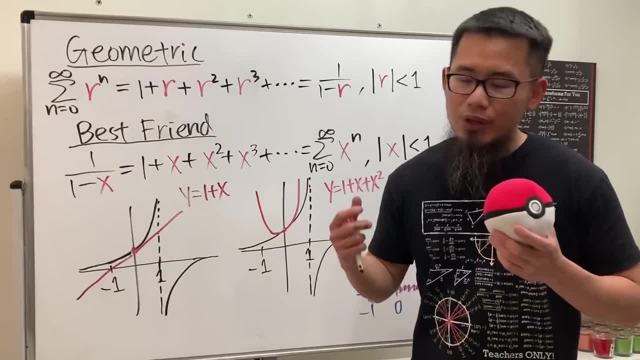 when you're trying to do computations with fractions or irrational numbers. that's it.